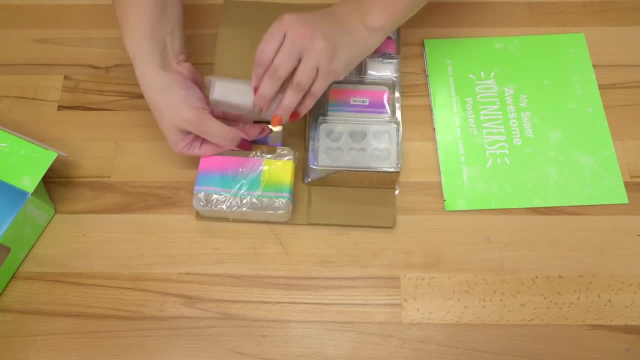 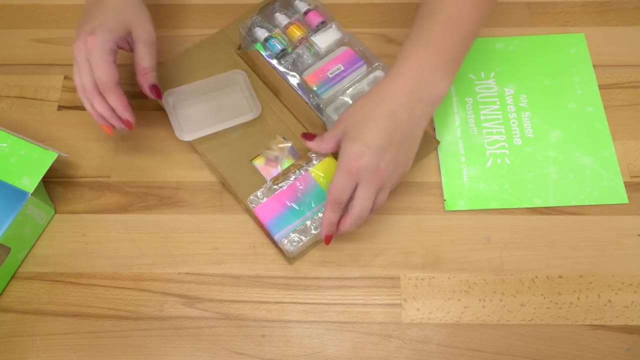 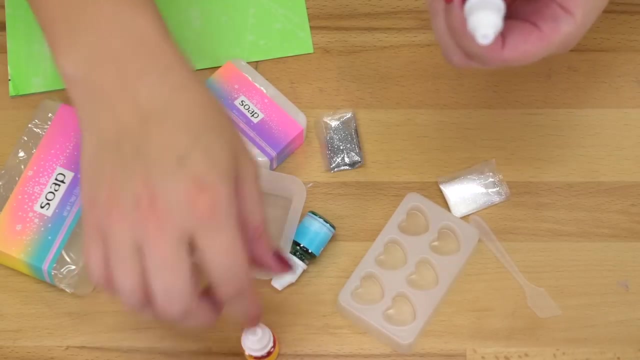 embed mold. Super cute. They have our little soap mold here and a little bit of melt and pour. Looks like this is a very clear melt and pour. This is about 10 ounces or so of melt and pour. I love the packaging. That's really cute. So we've got our colors. We have our little molds here. We even have 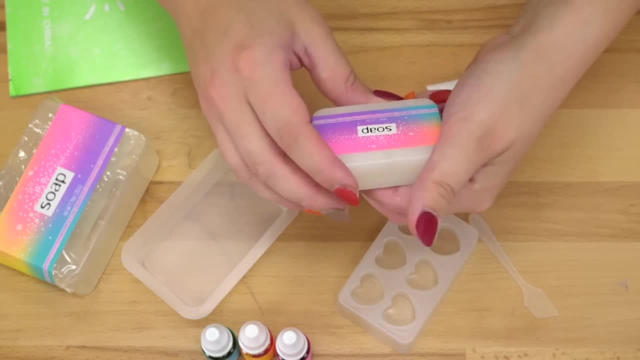 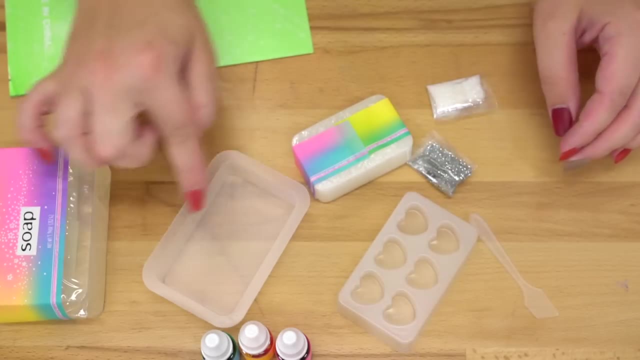 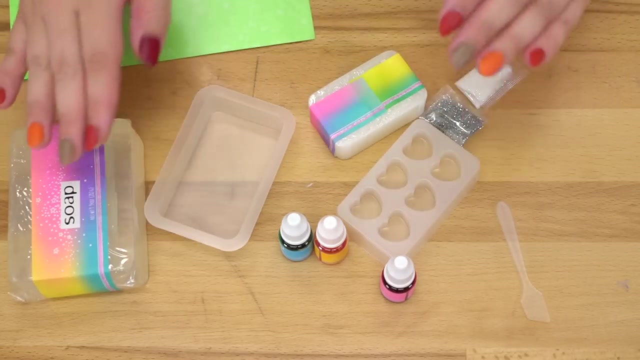 some special glitter, and our soap that looks like this is a little more opaque and this is clear. So this is for the surrounding area. Now, the one thing I'm not seeing in this collection is fragrance, and, as this is a kit aimed towards children, I'm hoping that the soap base is 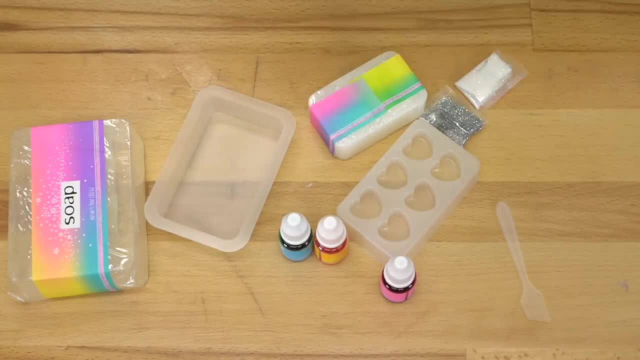 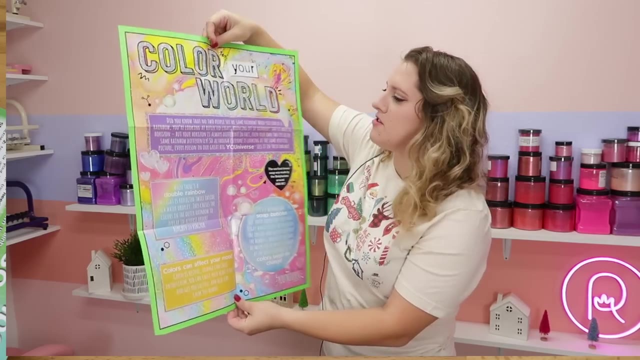 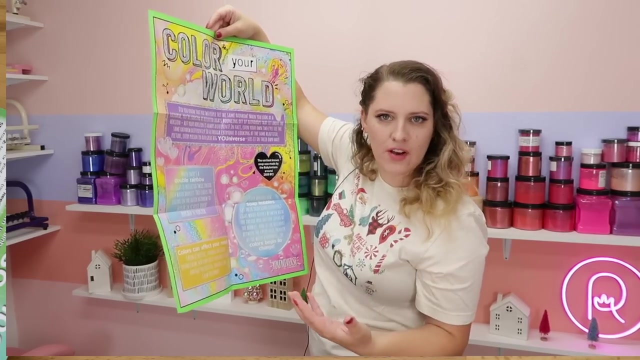 pre-scented, because that is something you just need. Here are my instructions, and this kit comes with a really cool little poster. On here are some soap facts like about bubbles and rainbows- Super fun. So we're going to start by adding some colors straight to these cells. They said you can. 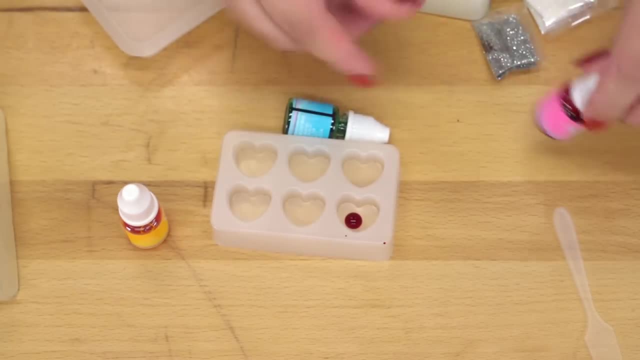 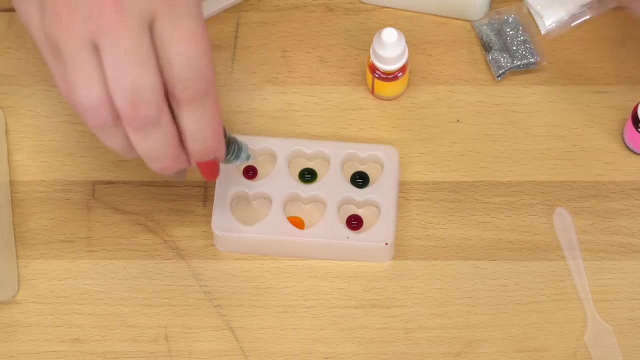 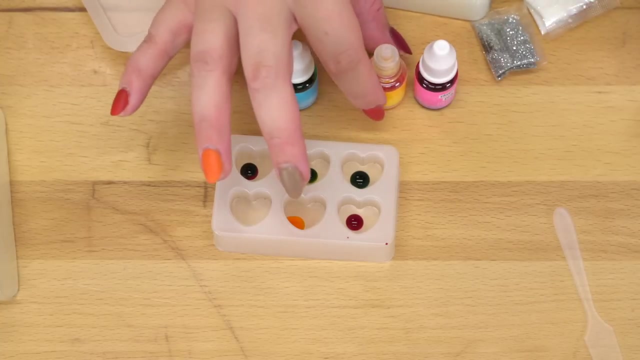 do up to three drops, So let's do that real quick and I think they're having you add it straight to the mold so that you don't have to use another dish, which is awesome. All right, I'm mixing everything up so that, hopefully, I get all six colors of that little primary rainbow here. I'm 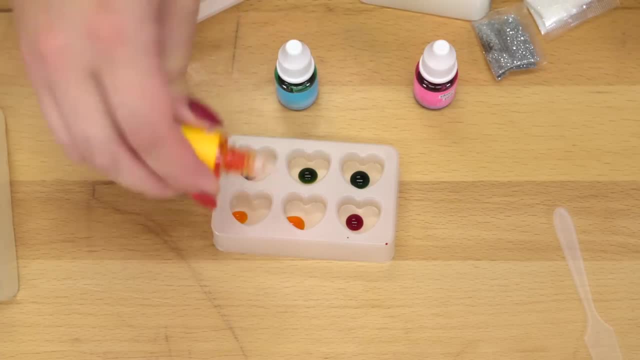 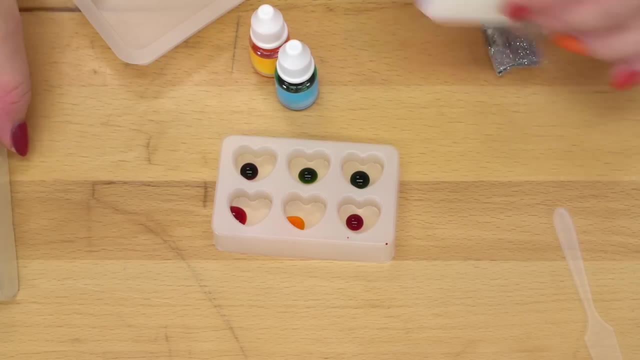 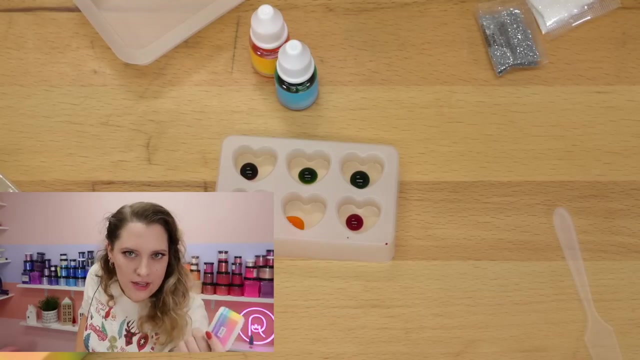 going to do two yellow and one red as our final color. Hopefully that will make some sort of orange and apparently, if I do everything right, I can make three soaps with this kit, So I'm going to cut this into thirds. If you're a kid watching this, 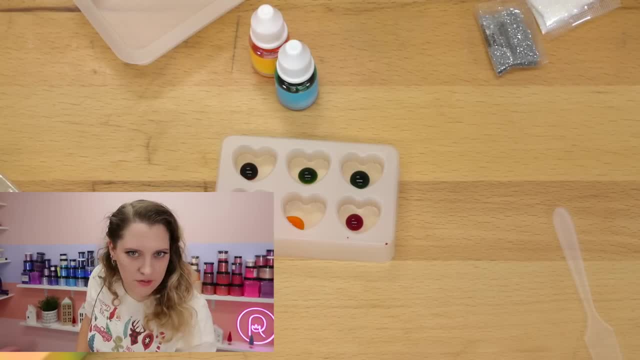 video. this is the part that you bring an adult in, for I hope there's no children out there making soap unsupervised, but just in case there is, have an adult or a friend older than 18 come in and help you with this. I'm gonna cut that here, I'm just gonna score it. 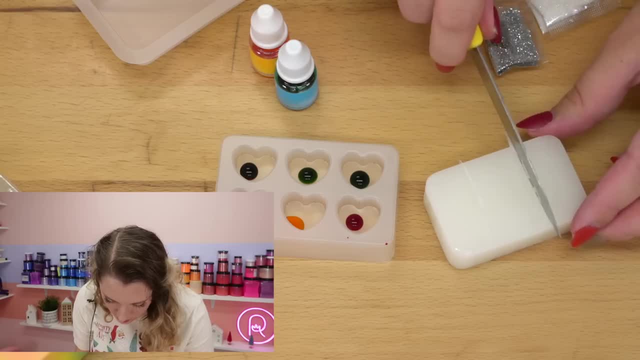 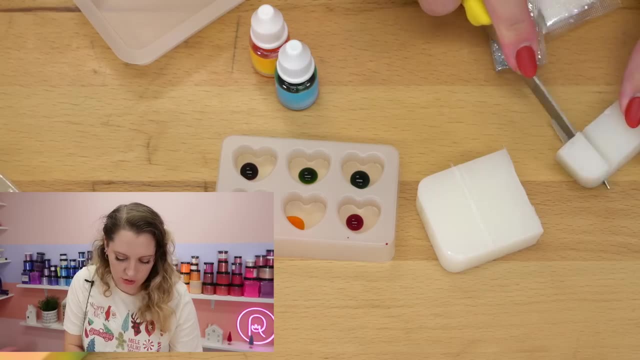 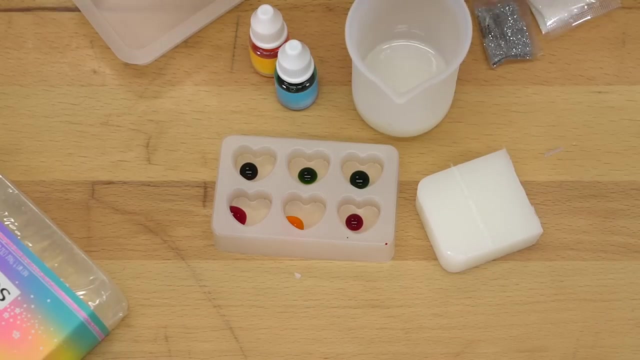 On these points so that I know approximately how much I need. That's about even right here. Just chop that, and then you do need a little container. So I'm gonna go get a little container. I'm gonna melt this down for about 15 seconds. Okay, it only took 10 seconds to melt that down. 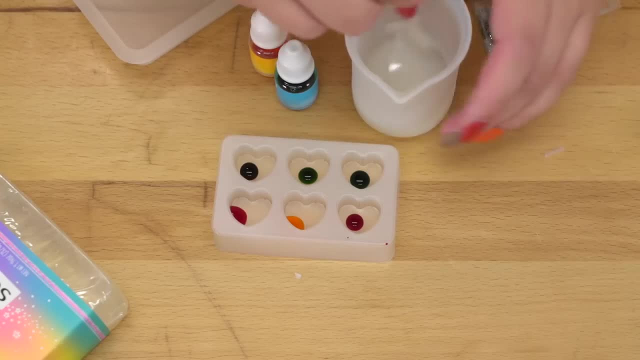 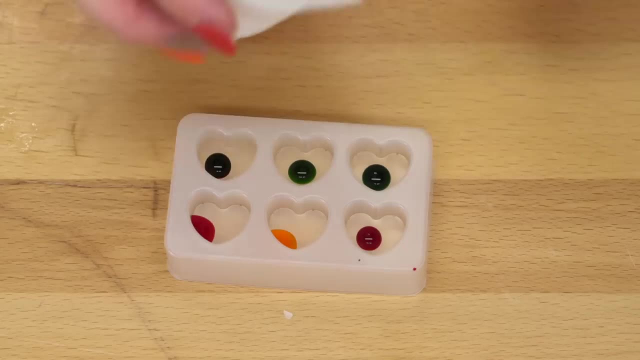 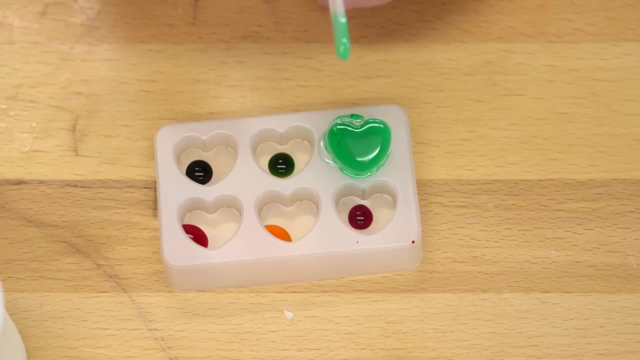 So almost no time at all, and it is quite warm, So I'm going to be careful when I pour this in to make sure that it doesn't melt the little plastic container. And then let's see how well we can mix it with our dye here. Very nice, So our blue is very green. 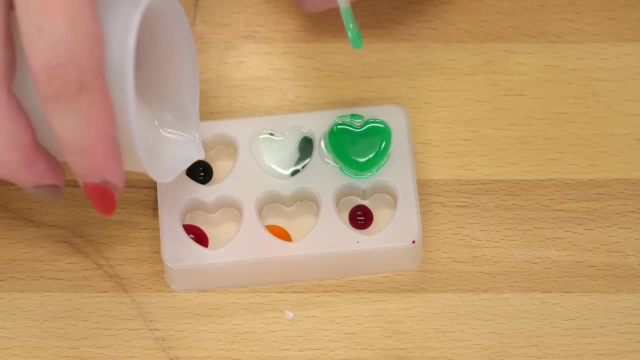 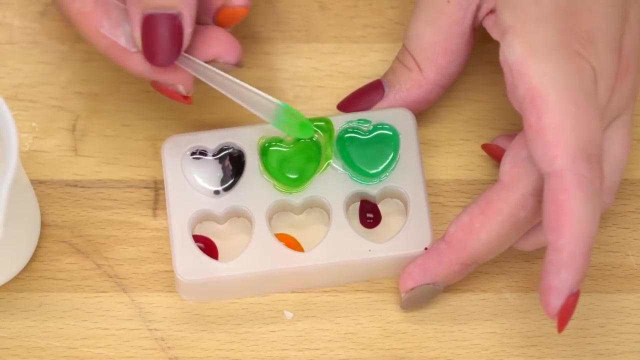 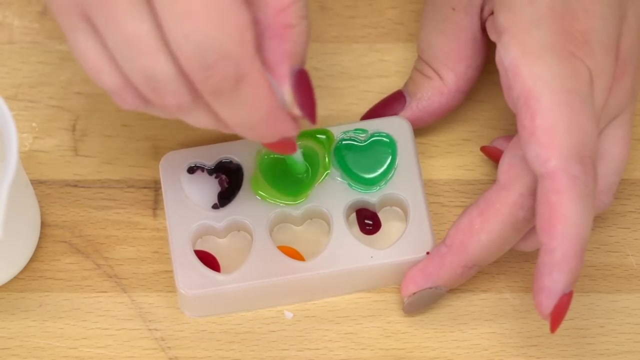 It makes me kind of wonder how green our green is going to be Very green, Okay, so the blue is blue by comparison. It is kind of hard to stir this in such a way that you keep all the dye and the soap in this tiny container. Maybe I need to get something smaller to stir it and I'd be better off. 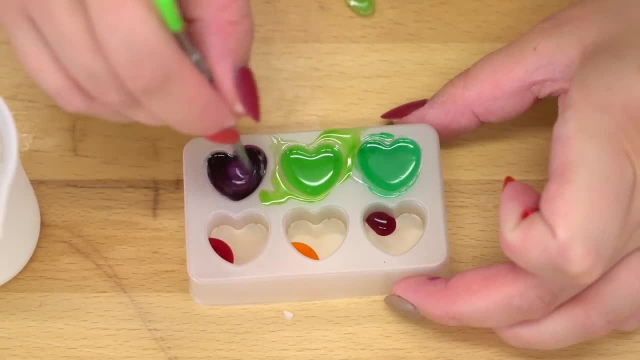 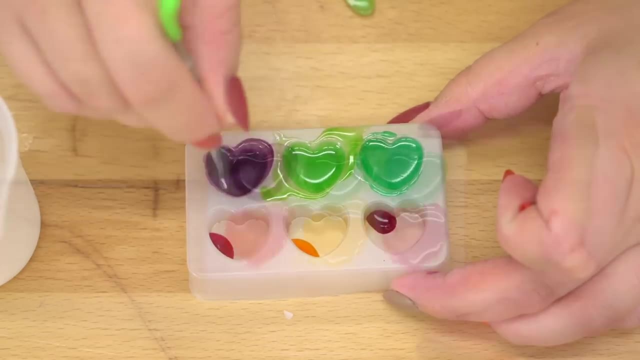 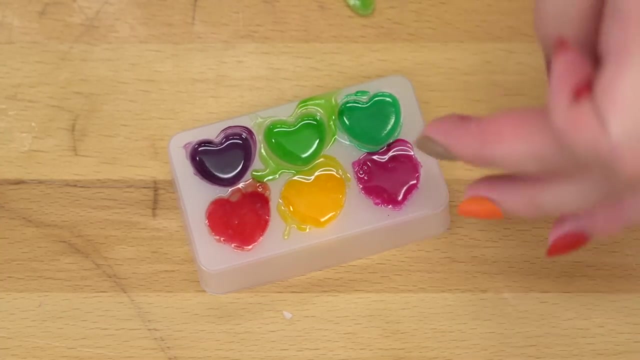 Okay, I went and got this little bowl. Oh yeah, that's much easier. Also, that's such a pretty color. I just want to make sure that the whole bottom gets colored Okay. so those colors are definitely vibrant. They're not exactly the colors that you see in the advertisement, but they're still really pretty. 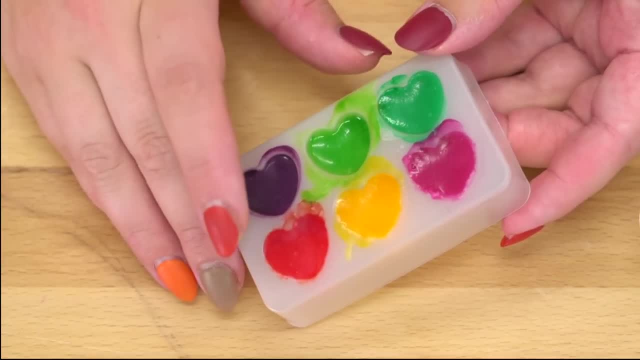 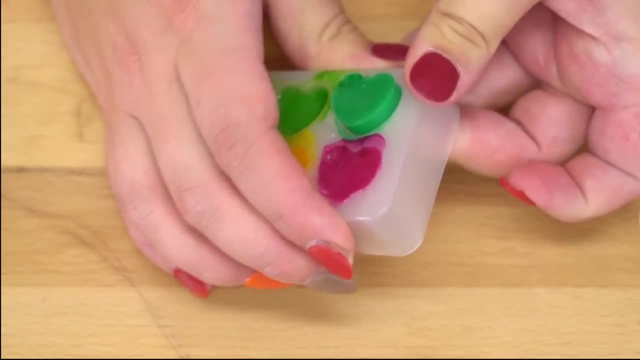 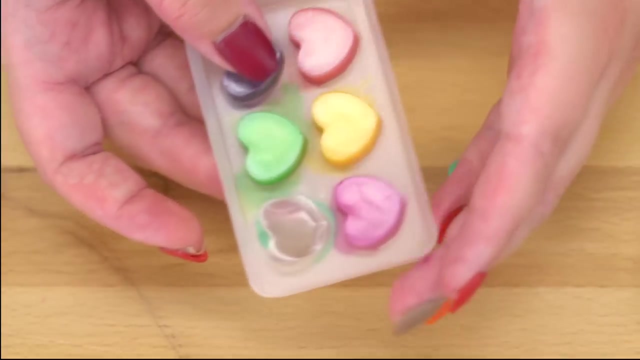 Okay, so I let this sit in the freezer slash refrigerator for, like I don't know, five minutes maybe. So now I'm gonna try to pop them out of the mold without breaking the mold. The mold is thin, so I would hate to dent it irreversibly, even though it kind of looks like. 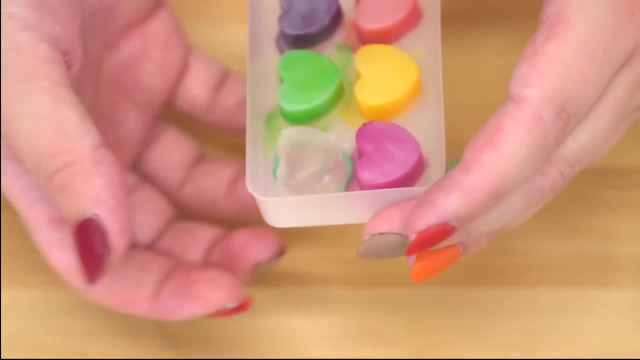 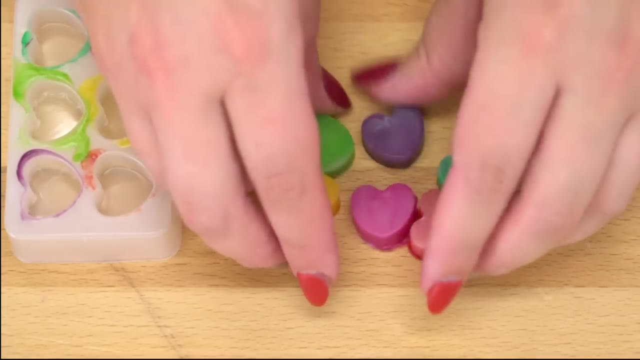 that's exactly what I just did. Let's see if it'll pop back out. Okay, all right, we, we've made a full recovery. Okay, all of them are out of the embed mold now, and I didn't quite mix this orange one up enough because it looks really good on the back, But then when you turn it over, you can. 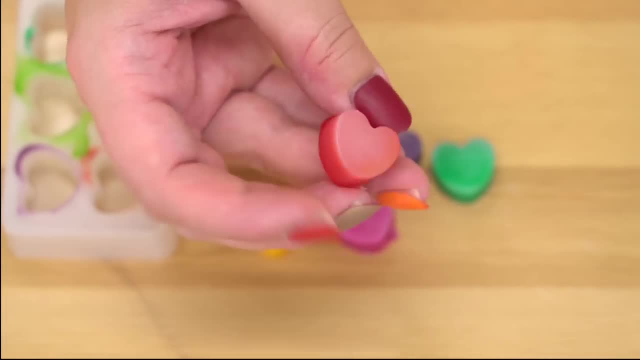 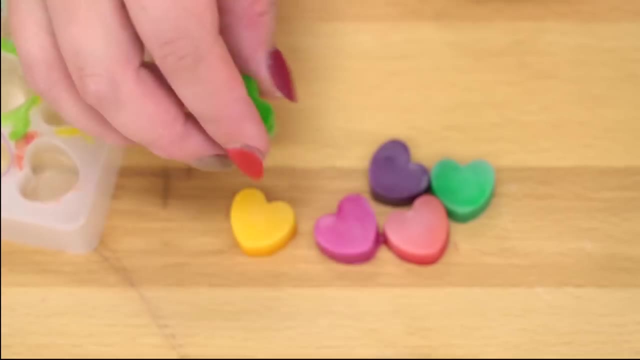 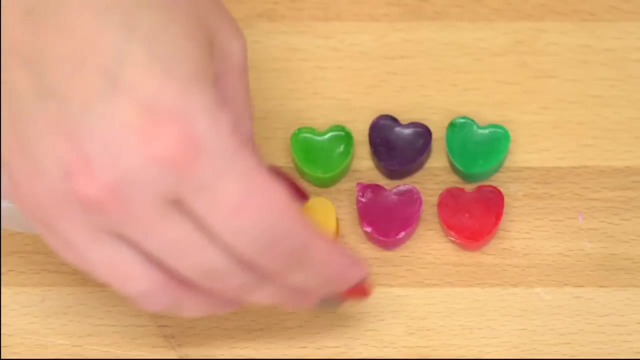 see, there's like a little gradient here where I didn't get it all the way to the bottom, But besides that, apparently I also did that to the green one, It's whatever- They actually all look really good. So I think what I'm gonna do is just place all of them, facing up like this, into my mold. Okay, let's. 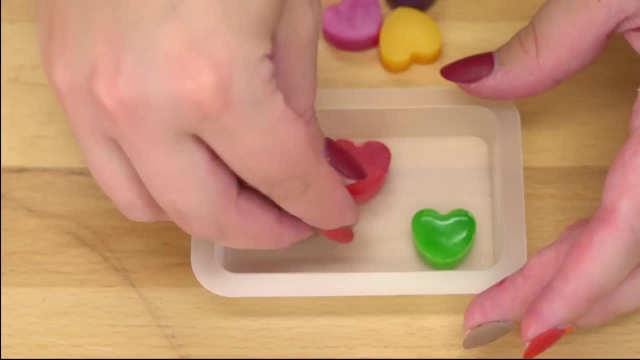 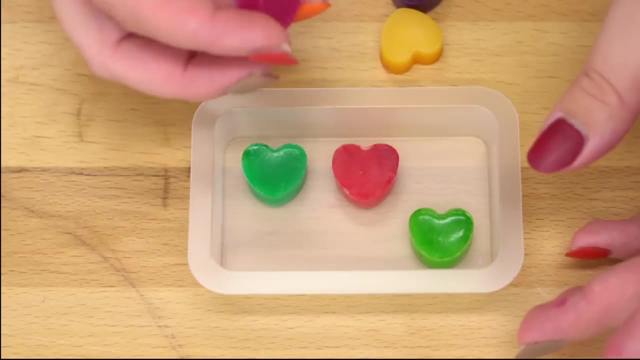 put them in, So I'm going to put these in a way that I think looks very pleasing to the eye. The green and the blue look the most similar, so I'm gonna try to separate those. Okay, this is looking really good. Hopefully, it's not all the way to the top, So I'm gonna put the green one on top You. 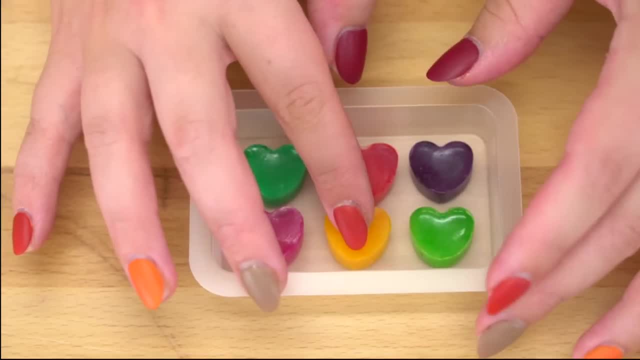 guys can see what the top looks like here, and then I'm also gonna put the pink one on top. It's just kinda like my third eye, So it's kinda like a little bit here and then there's just a little bit. they'll stay in place. whenever I pour that first layer, Let's go and melt down our clear melt and 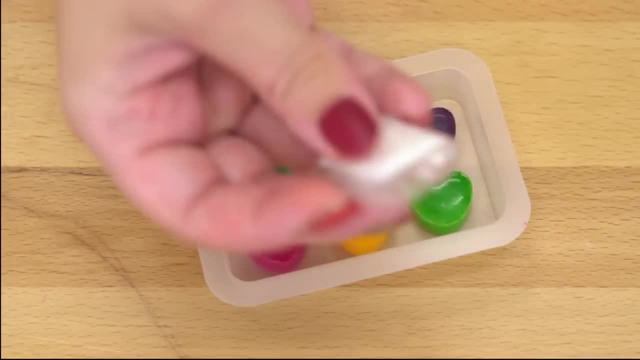 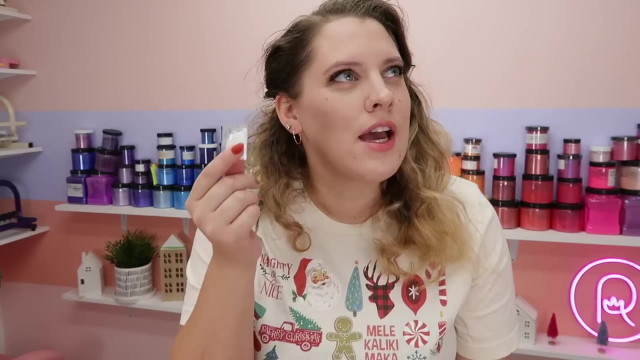 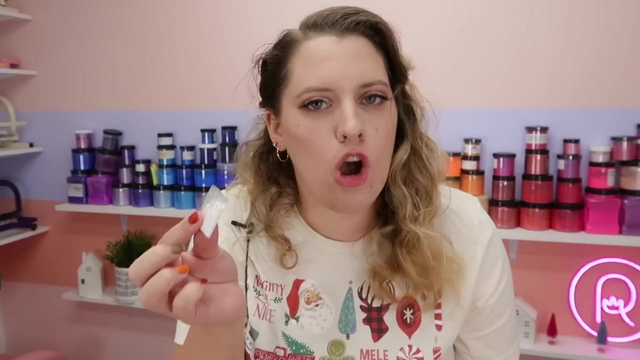 pour soap base and add a little bit of this glitter to it. A note about the glitter: It is probably not eco-friendly. Okay, that's something people typically advertise, So it's probably made out of plastic. We hope for improvement in the future. They will switch over. We have high hopes. 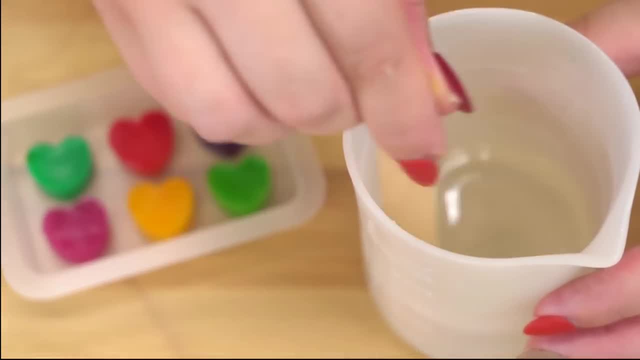 for that. Okay, I admit it, I am using a popsicle stick. all right, I'm just not going to use that teeny, teeny, tiny little stirring spatula. okay, Okay, I'm going to add just a little bit, just so. 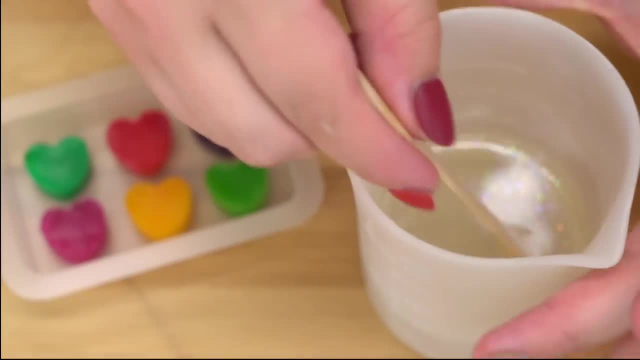 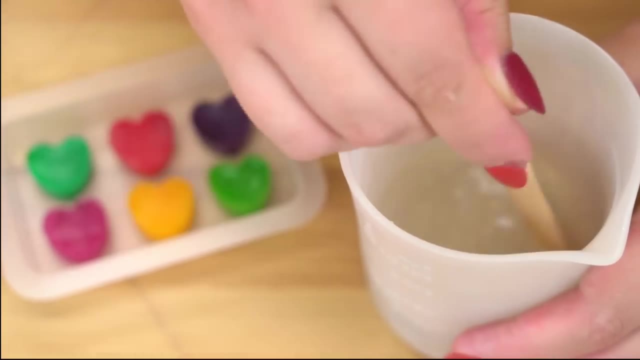 that we can see how it works in the other soaps. I won't be adding any of that glitter, but we do kind of want to get an idea of what it feels like in the soap, because I also have a little bit of a suspicion that it may not be cosmetic grade, It might just be a craft. 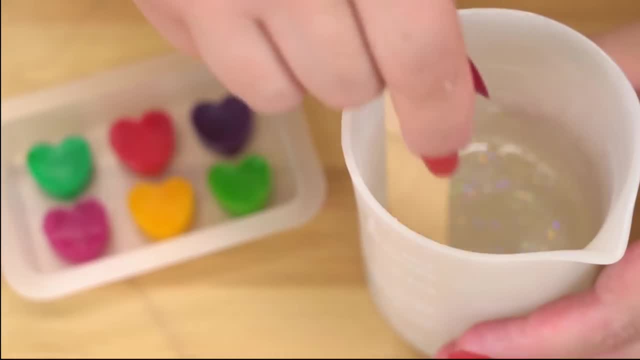 glitter, in which case it might feel scratchy on the skin, And I want you guys to know that. if it is So, that's why I'm adding it to this one, And that's right. I'm adding something else in, I'm 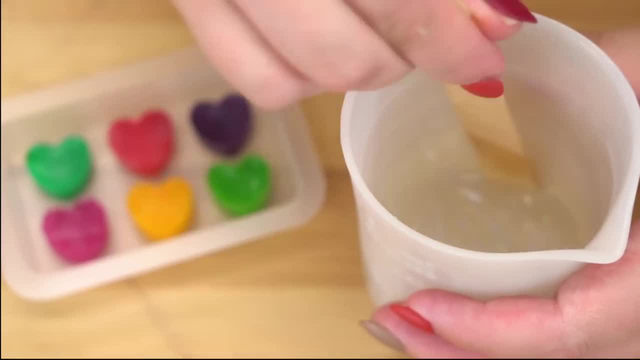 spritzing with rubbing alcohol. Rubbing alcohol is such an easy thing to add to a kit. I don't know why more kits don't have it, because it really does make a very big difference with how your finished product looks. Now, I've tried to let this cool a little bit so that it won't be 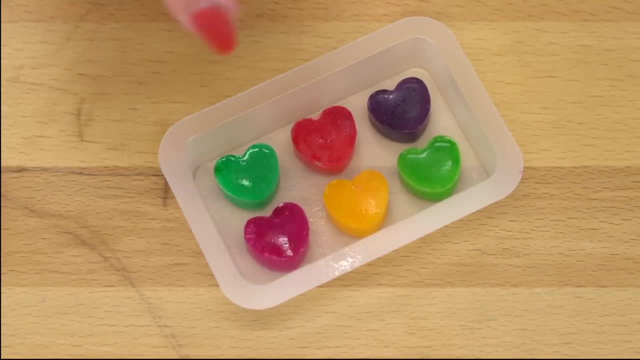 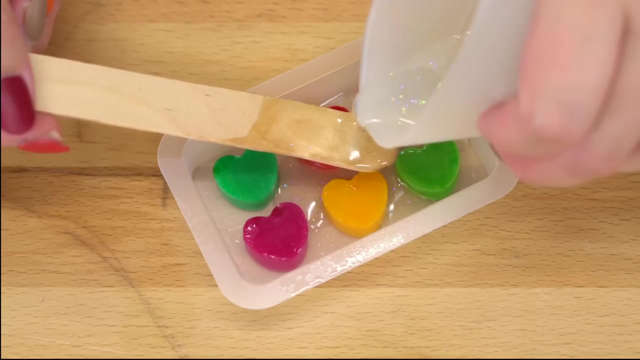 so hot when I pour it onto here. But I'm also going to spritz these with rubbing alcohol so that hopefully they grab a hold of this soap And then, hot tip, use whatever pouring or stirring utensil that you have to break the fall of your soap so that it fills around nice and slow and 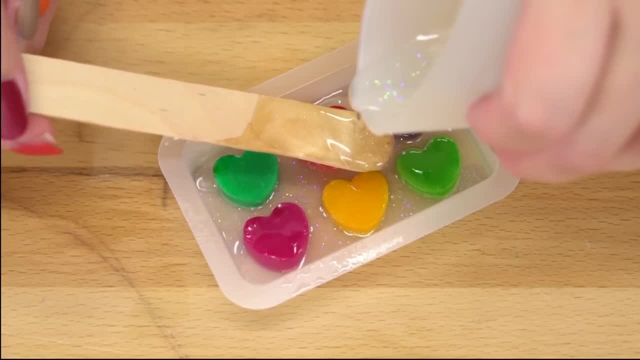 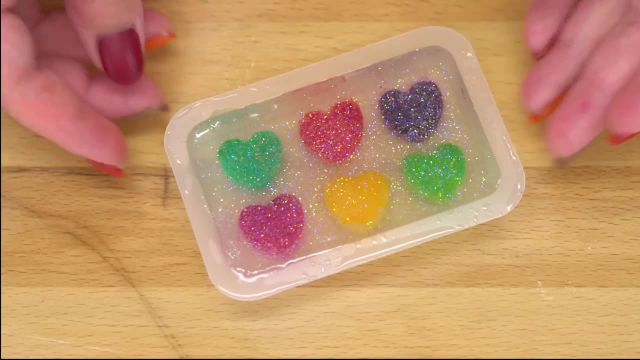 doesn't move your embeds around. That is what I like to do And it has worked very well for me in the past. All right, now I'm going to spritz And we are going to let this set up completely before we. 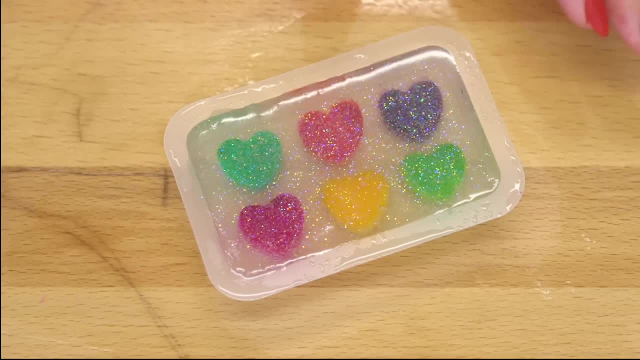 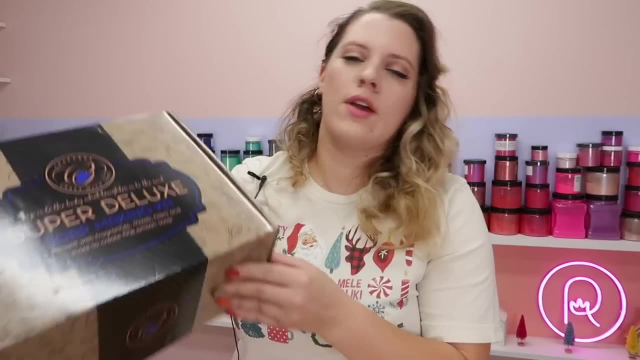 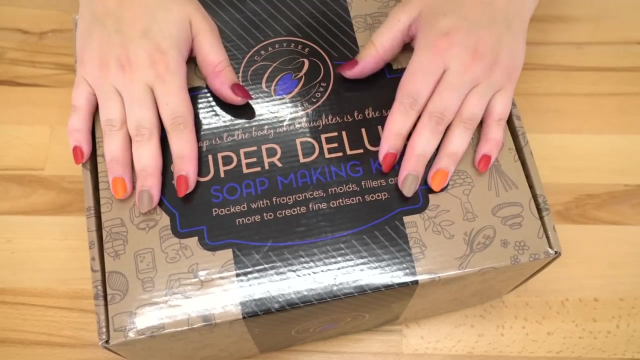 demold. Based on how hot everything was and the instructions, I'm going to bet this has to sit for about 30 minutes to an hour before I can take it out. Okay, so let's talk about the super deluxe soap baking kit. Really nice packaging. I will say that this print is upside down, But the box. 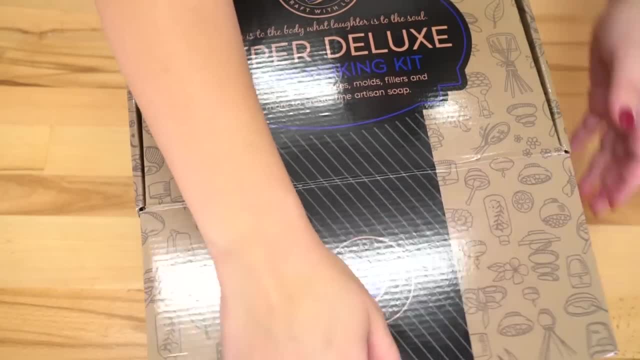 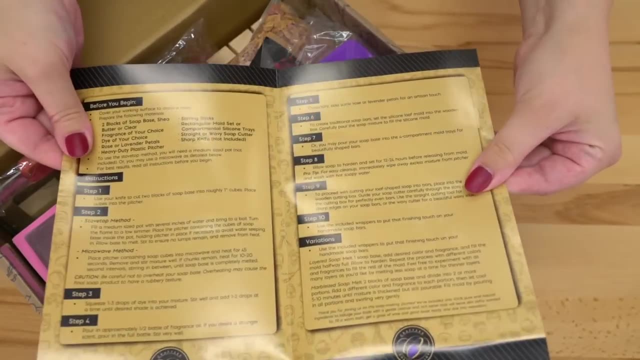 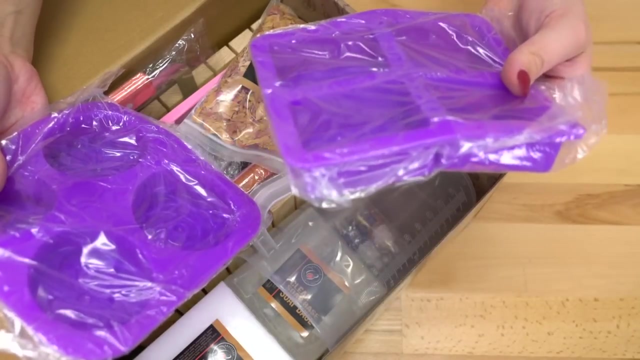 thing fell out during shipping, So let's go ahead and open it up. Oh, okay, All right, So there's a guide to soap. making no pictures, but that's okay, I'll forgive it. Look at these- so beautiful molds. 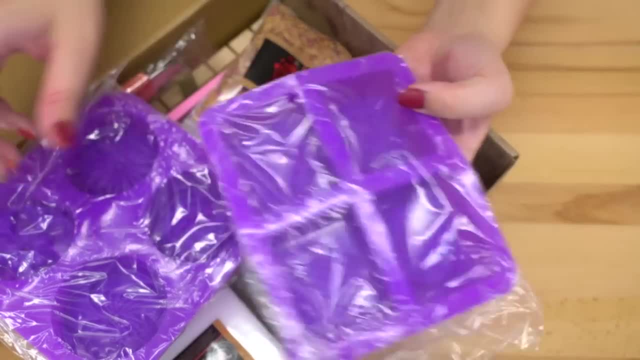 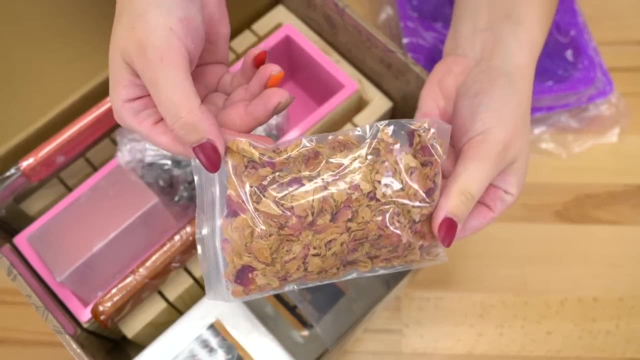 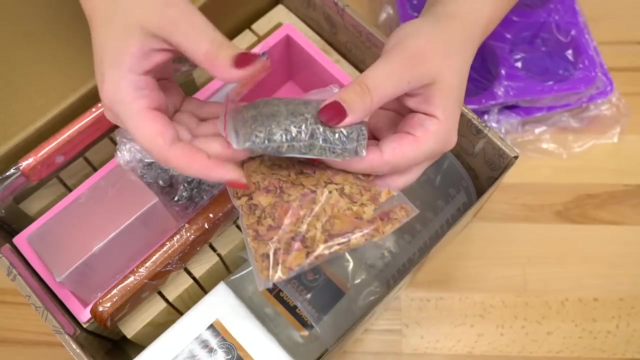 Oh, hold on though. I love this. I love it. That is so pretty. It comes with some botanicals looks like these may be on their way. I would hope for roses. you would see something a little more punchy, But the lavender, That's all. 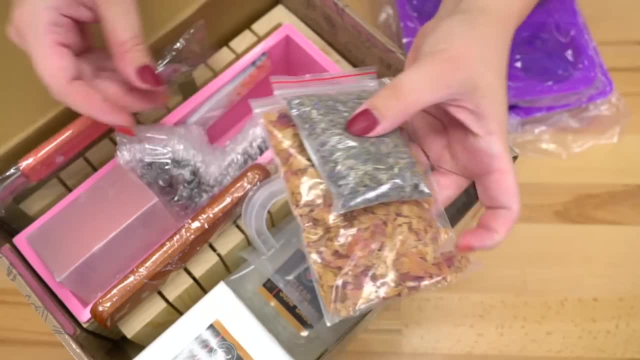 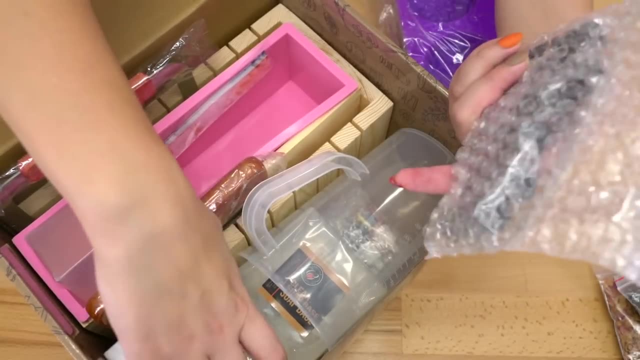 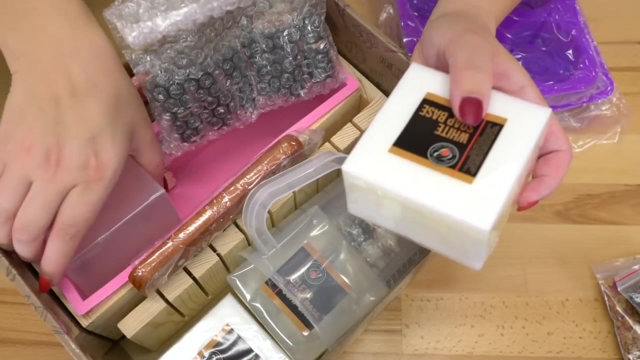 right, That's about a medium blue ish. It's not the most vibrant, but it's certainly not the most brown I've seen. Looks like we have some. What are these essential oils? Yeah, fragrance oils. We have melted poor. They even gave us a cutter and a loaf mold in case we wanted to try some loaf mold soap. 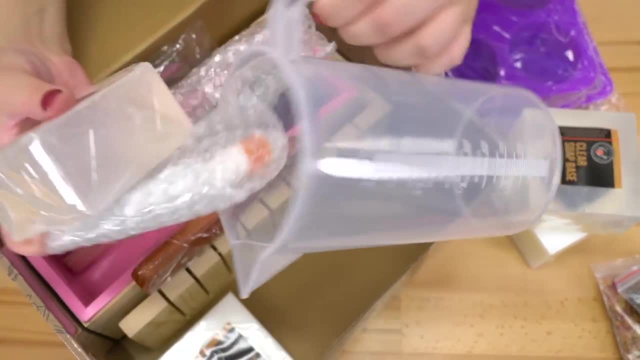 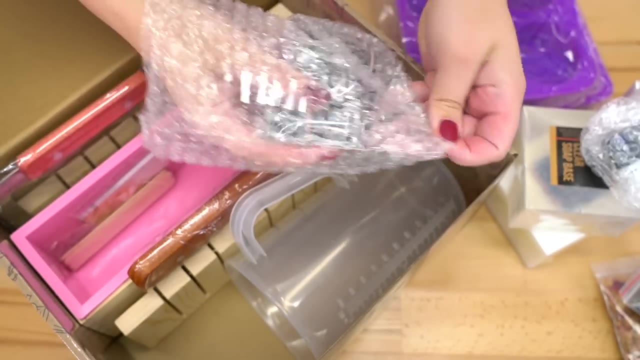 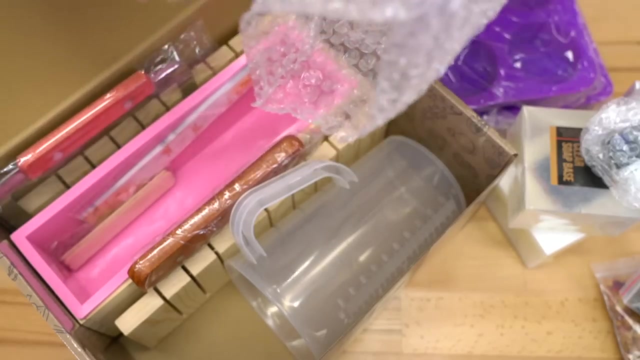 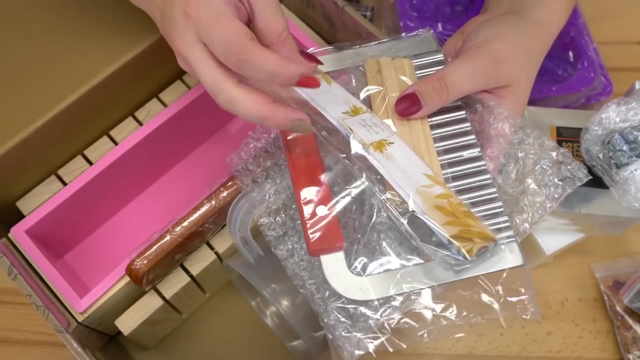 making. So this is a very, very complete kit. It comes with six different colorants. I bet these fragrances are good too. I can see some of them. We've got blueberry rose- looks like sunflower, orchid, cherry and a vanilla soap cutter. We have some popsicle sticks for stirring, Wow. 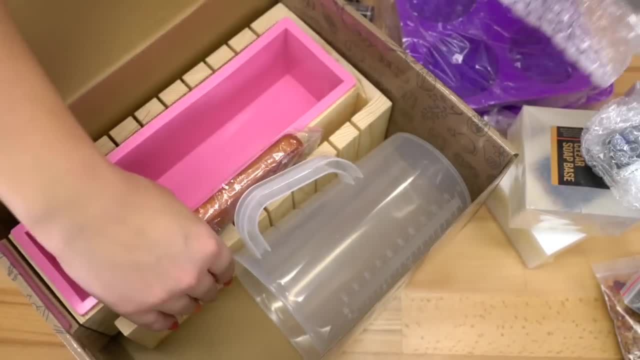 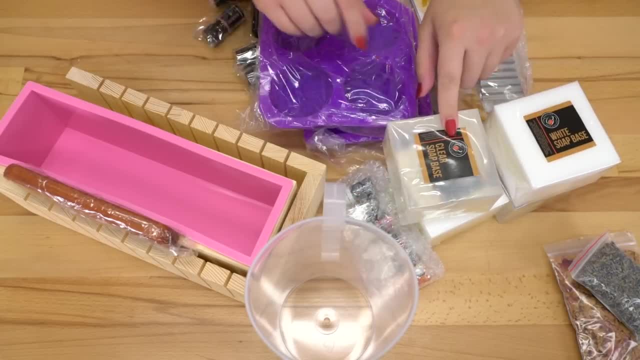 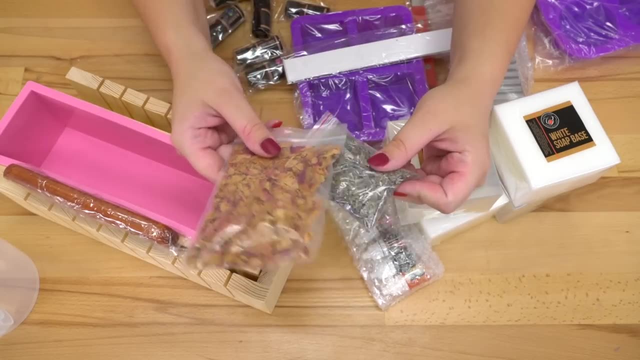 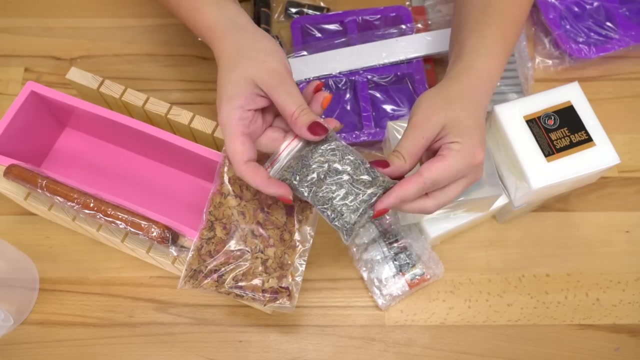 Now we have about four pounds of melted poor and they have the ingredients of the melted poor listed right here Now I personally do not recommend using botanicals with melted poor. They will turn very yucky colors, roses will just turn more Brown and the lavender buds will turn very brown and end up looking a 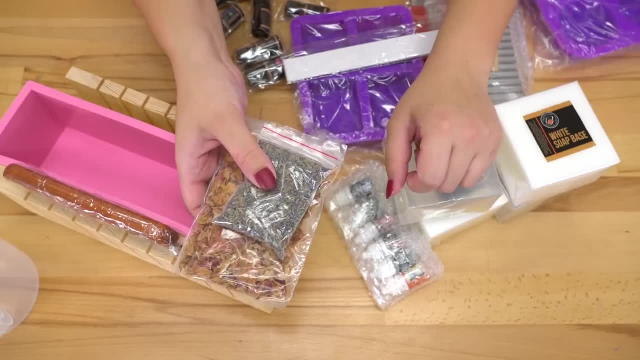 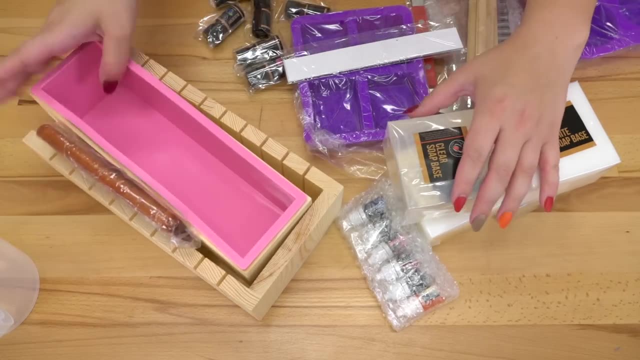 little bit like mouse droppings. So I'm going to discard these because these really, in my opinion, should be used as toppings on cold process soap and not melt and pour. so I'm going to set off to the side for future projects, But this is exactly the mold that I purchase and recommend for. 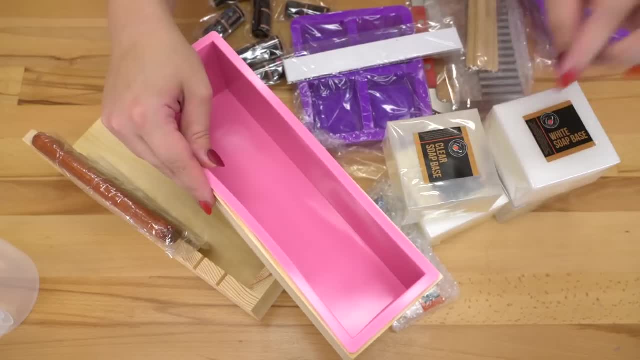 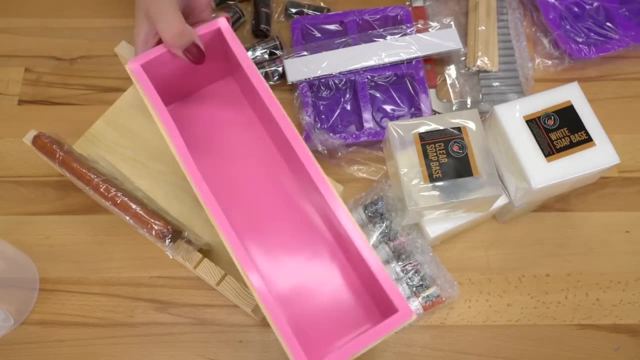 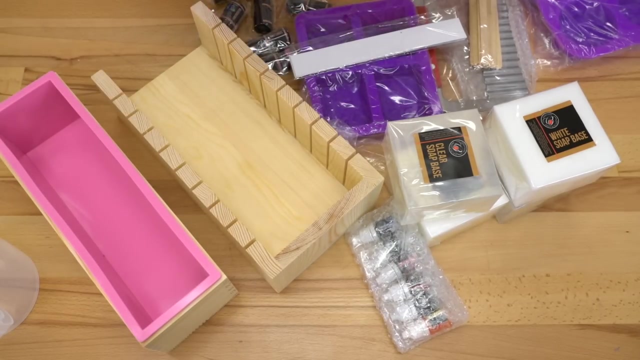 beginner soap makers for cold process soap. So if you wanted to dip your toe into melt and pour and then switch to cold process, you would already have the loaf mold that I purchased, and it's worth about $12 or so, So that's great. Then we have our little cutting setup here. So me personally, 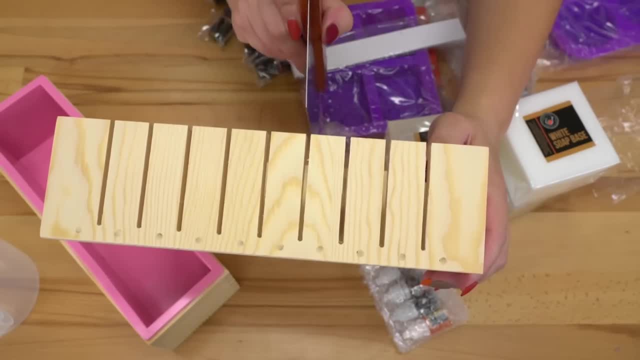 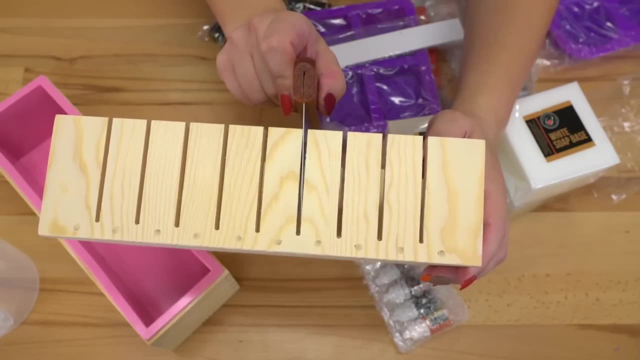 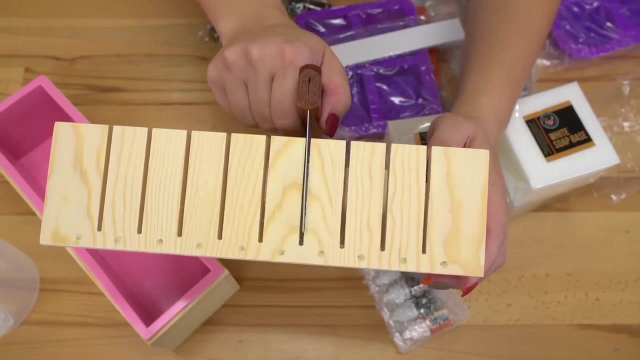 I have never had that much luck with these types of cutters, because when you slide this in, you can see that there's still about a millimeter or two of wiggle room here, And so I will like put it on an angle, and I will still make uneven cuts. Now, this is just me. It could work very, very well. 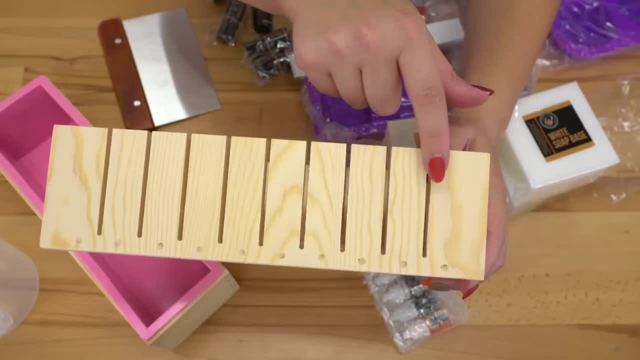 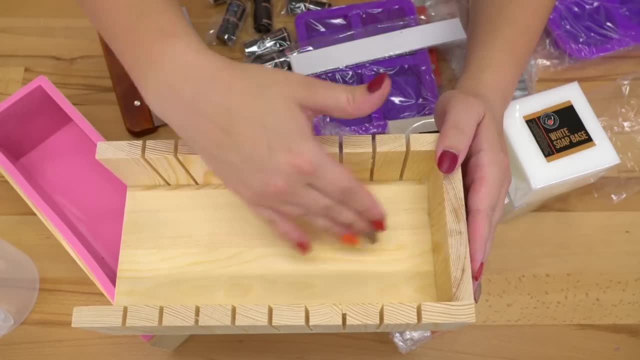 for some people. I do notice that in between these cuts here it has not been sanded, So that would be something to look out for, And it is unfinished wood. So if you cut a lot of sorts of different collectibles, you can see that there's still a little bit of wiggle room here. 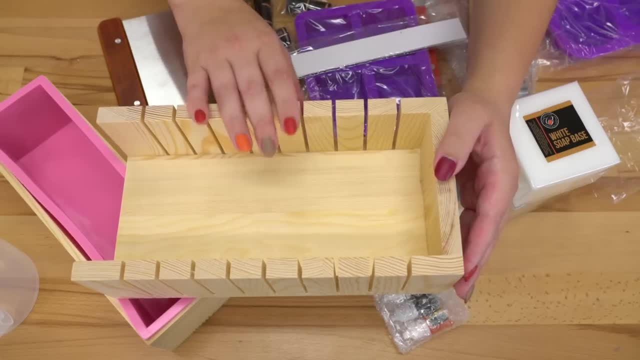 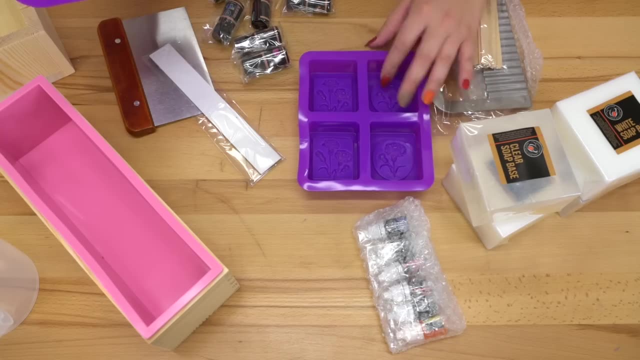 So that's something to look out for. And this is unfinished wood, So if you cut a lot of sorts of yourselves soap on this, There is going to be buildup. You're going to have to wash it. It would definitely be something I would recommend sealing before you use. Maybe we can do some pretty stuff on these. 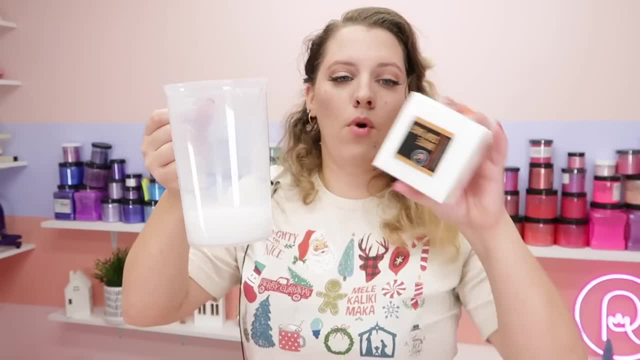 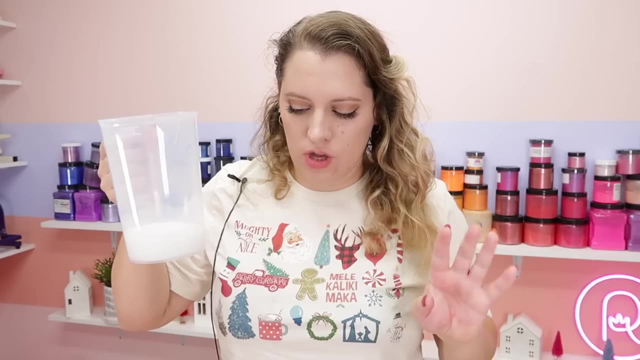 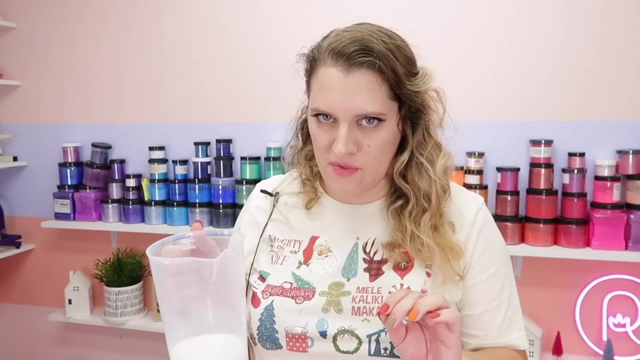 flowers here. Okay, so I have melted down one half of the white soap blocks. So at this point I think I'm just going to try to cover the bottom of all the little purple silicone molds and then we'll go from there. I'm not going to add any color or fragrance to this, I'm just going. 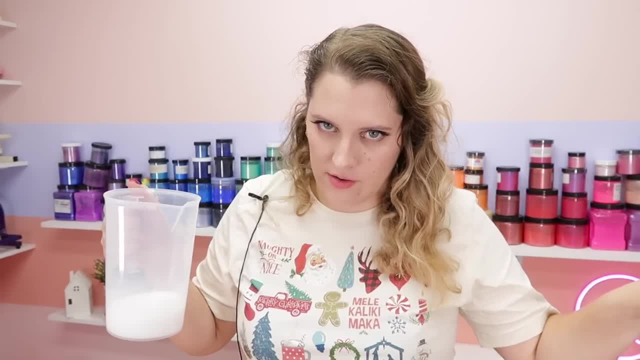 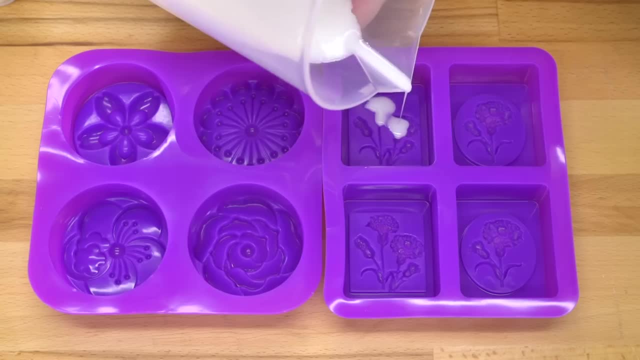 to color in those flowers. then we'll think about coloring and fragrancing. This is a pretty specific pouring tip, so I feel like it's going to make my job a bit easier. There are some extremely fine parts of this mold, so if I overlap a little bit, that's okay. I just want to make 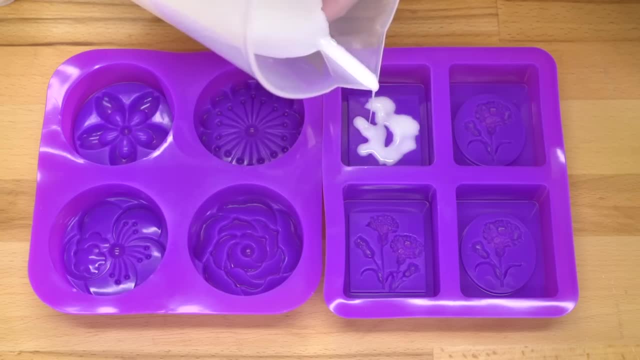 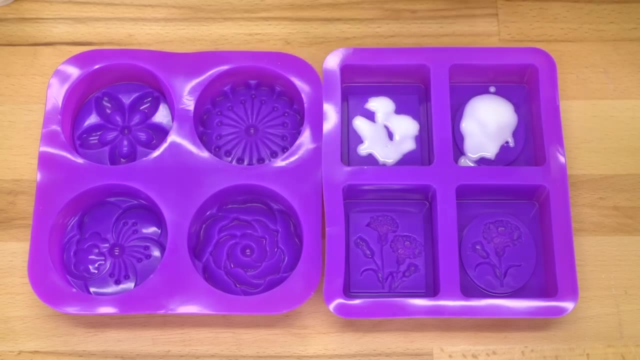 sure that the flowers themselves are covered And everything has gotten into those cracks. so that's fine, right there, That's whoops. Well, that's not the most ideal, but the other one was. Maybe I can just move it around with one. 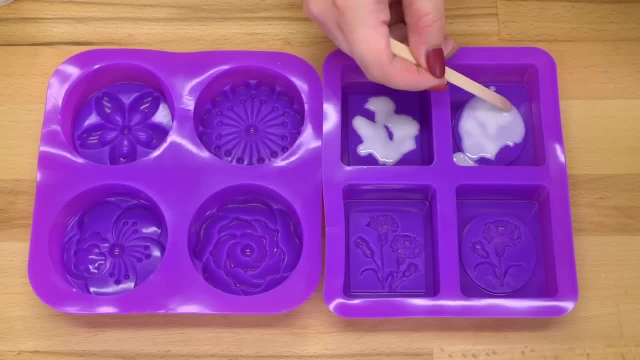 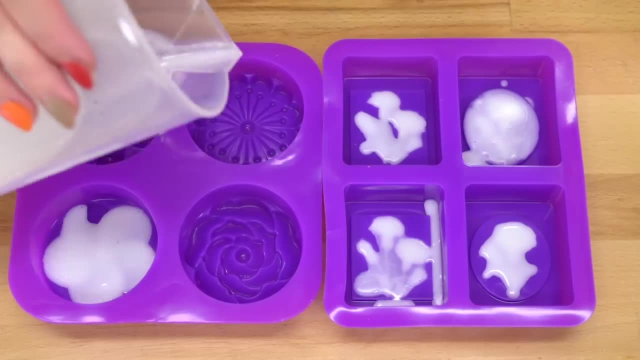 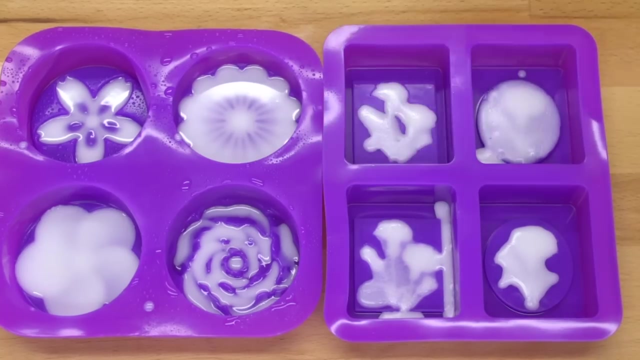 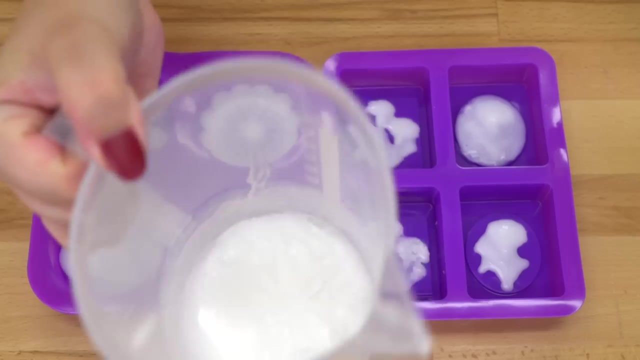 of the popsicle sticks like right to the edge, like this. Okay, with all of the white done and everything kind of cleaned up a little bit, I am going to melt this down a little bit more because it's starting to thicken up. Okay, I think it would be really. 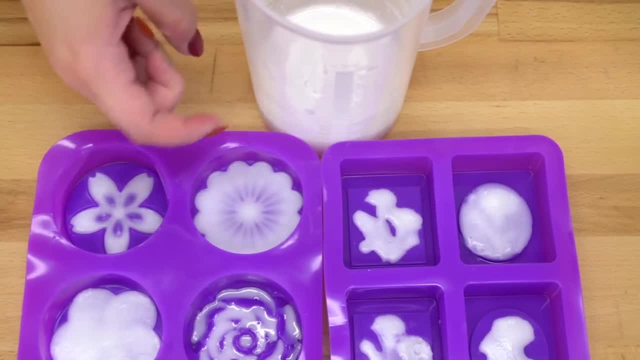 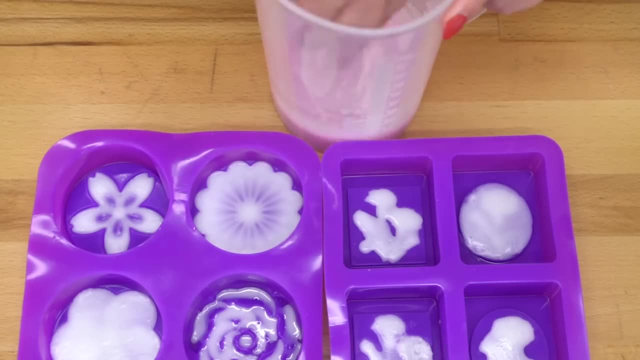 nice for this first set here if we did pink in here. Ooh, okay, so pretty pigmented actually. Yes, yes, very pigmented. One drop goes a long way. I'm going to give it a spritz, but I'm also. 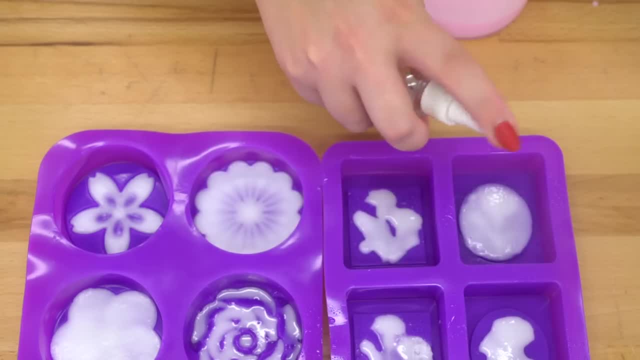 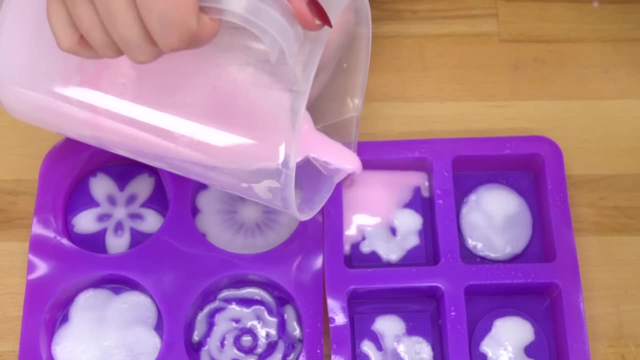 going to spritz my molds and this white soap block. I'm going to give it a little bit of white melt and pour that I poured in first. Now I don't know how many I'm going to be able to fill up with this and I am just going to pour in the corner, so we'll just have to see. Okay. 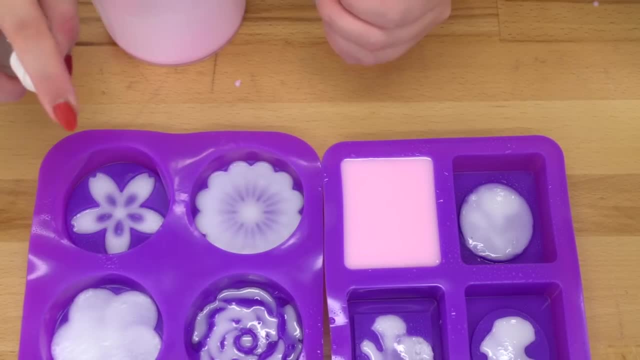 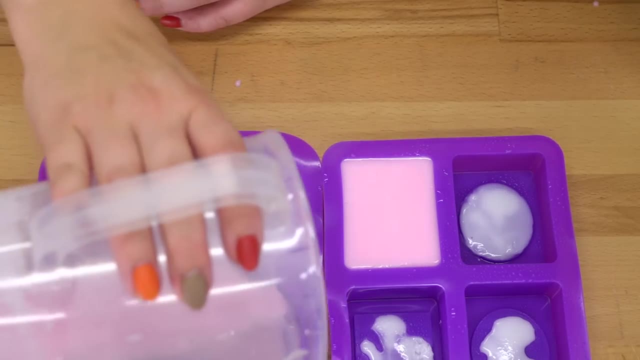 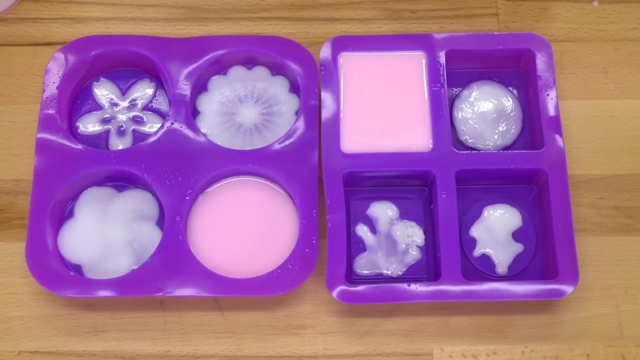 the rest of it. I'm actually going to pour into, I think, the rose, because I don't have enough to do the other soaps and I think that'll look really pretty with the rose. I'm just going to get all of that into there. Okay, then I'm going to cut up this other half and I'll fragrance it and 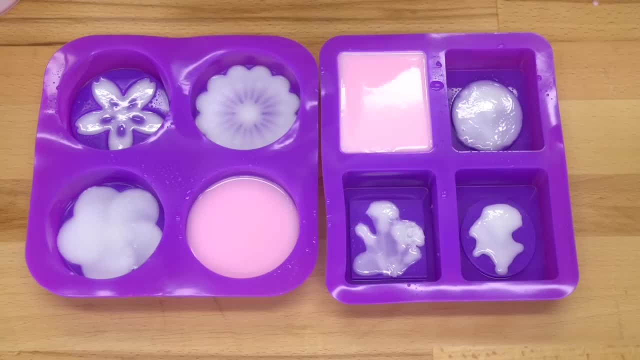 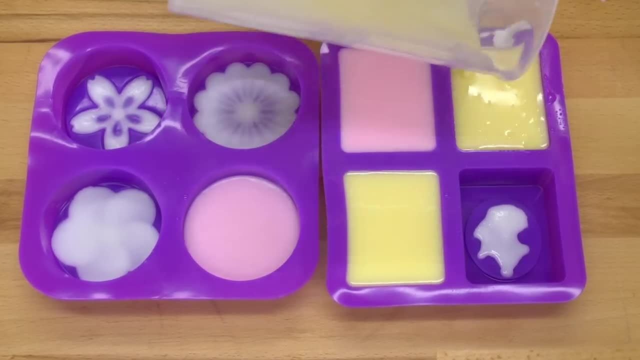 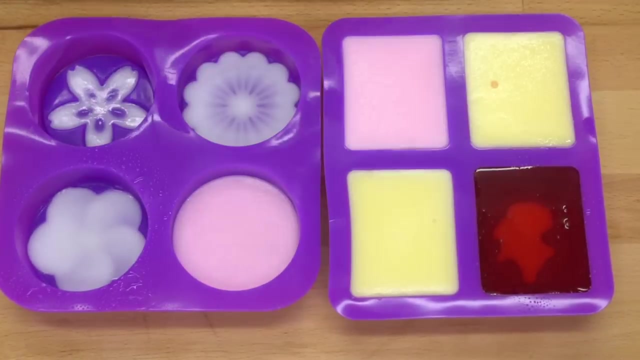 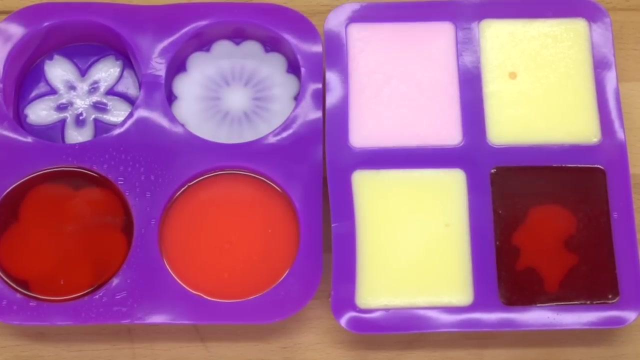 color it. I'm going to do a little bit of a white melt and pour that I poured in first. Now I'm going to color it a bit differently and we'll start filling in all these other cavities as well. So I am getting ready to pour the final. 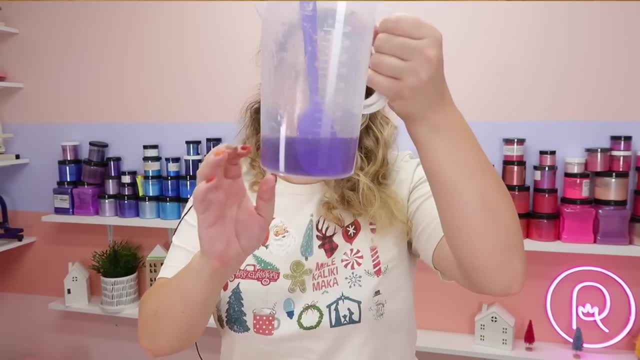 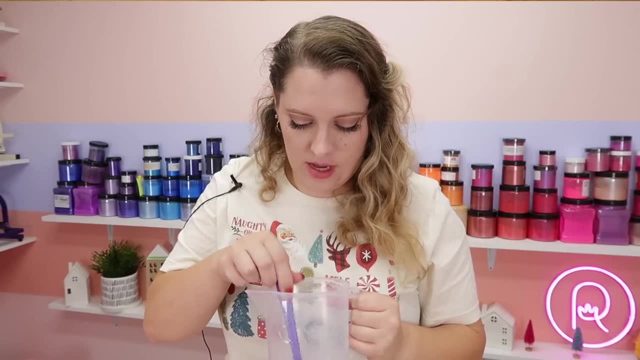 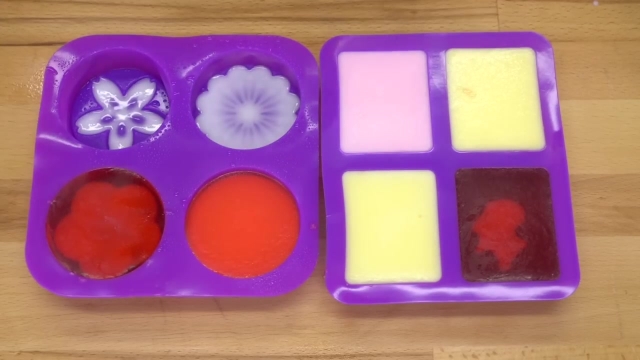 soap color for the silicone molds. This is the purple, and I added the vanilla to this one, so it's going to be the one that I watch over the next couple of days to see if it turns brown over time. I'm going to spritz these with some rubbing alcohol, and probably this one too, because I think 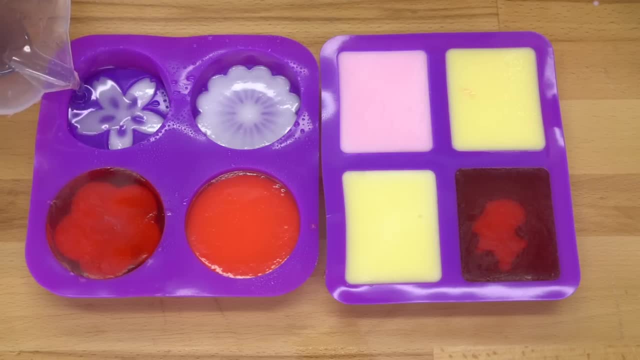 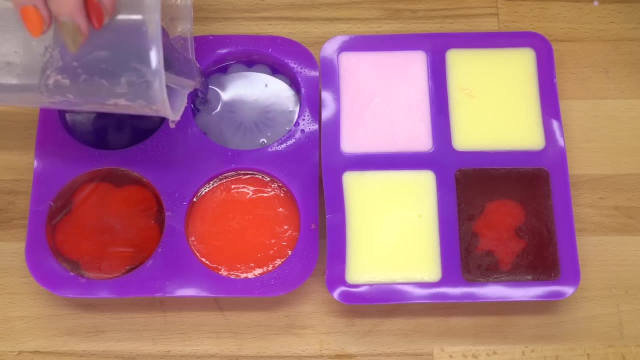 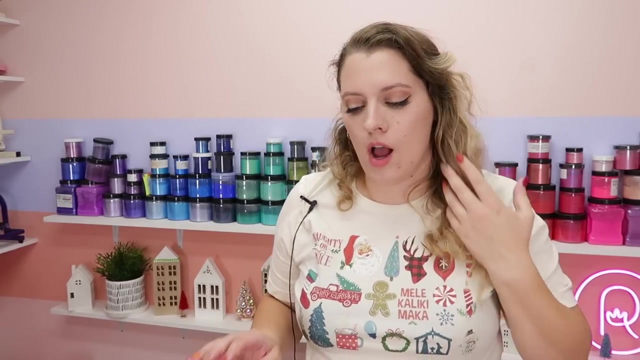 I might have a little bit left over. Then we're just going to start pouring it in just like so, Pour some more in, All right, everything looks super good, and these have to sit for quite some time before I can move them. 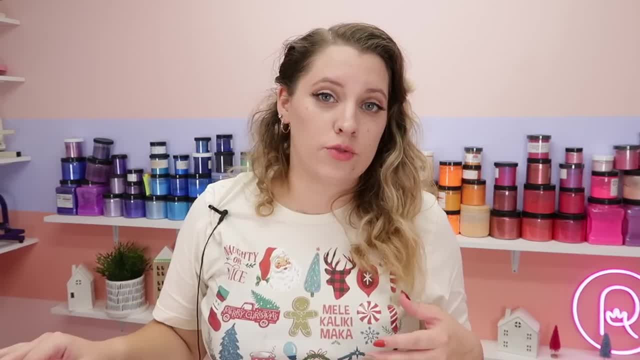 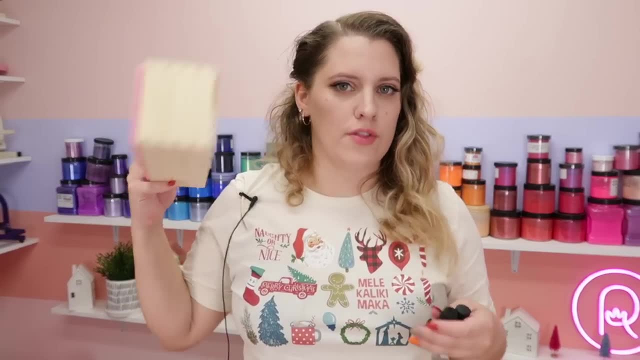 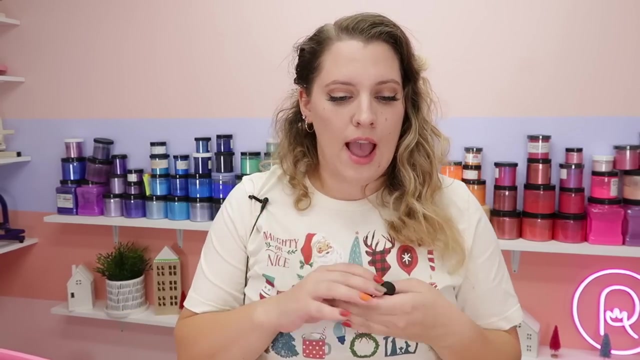 before I can unmold them. The instructions recommended 12 to 24 hours. So I think what we'll do is we will use the loaf mold for the last bit of the melt and pour in this kit. We will fragrance it with cherry and with the blueberry and we will do it blue and white maybe. 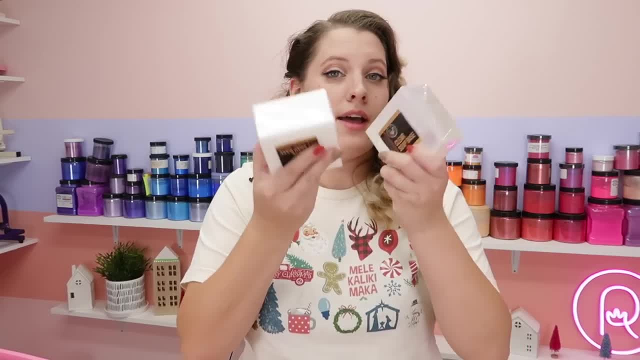 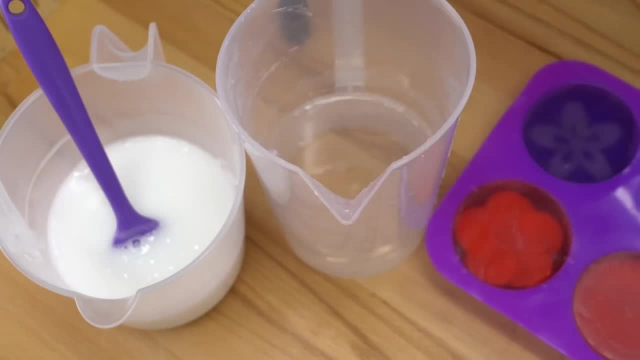 I think that would look really pretty. So I'm going to go ahead and melt down both of these blocks and then we will pour it into our loaf mold. All righty, so we are putting the entire cherry fragrance into the white. Oh, it kind of smells like cherry medicine, not gonna lie. 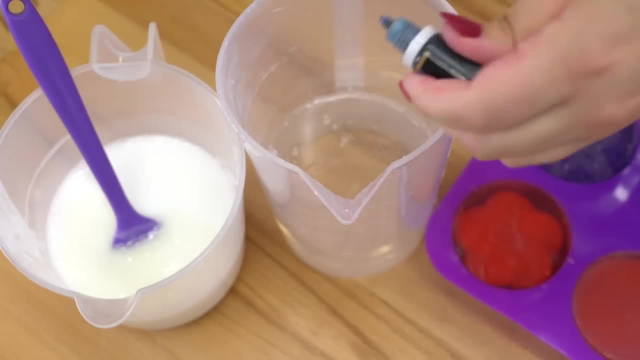 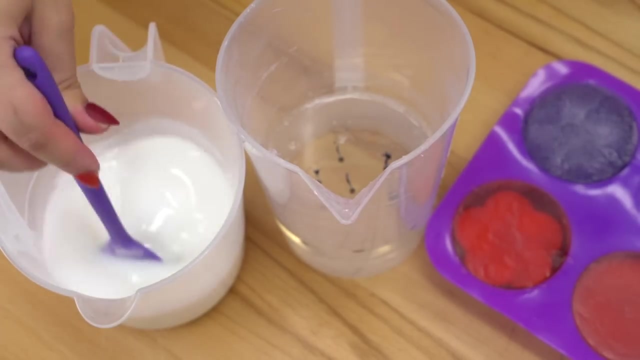 And then the entire blueberry one into the clear. Like I said, the white is going to remain uncolored and then the clear is going to be blue. So this is the last time I'm going to stir the white, So I'm going to make sure that I wipe down all the edges, Okay, 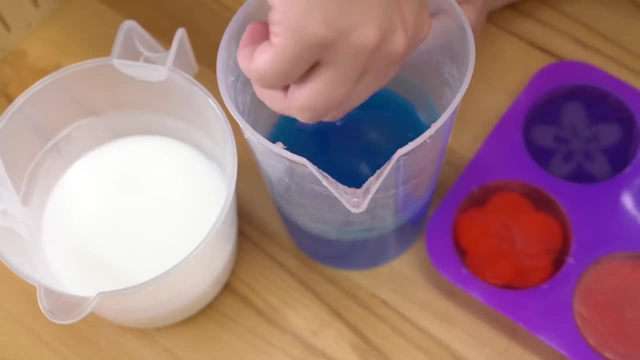 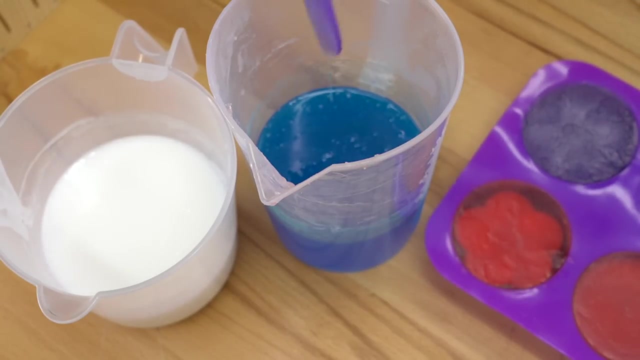 and now for the clear. This one smells a lot better, in my opinion. All right, and then I'm going to let these cool down a little bit. They're kind of hot right now and I feel like if I mix them together they may blend too much. I don't know, I don't know. Let's go ahead and test it. 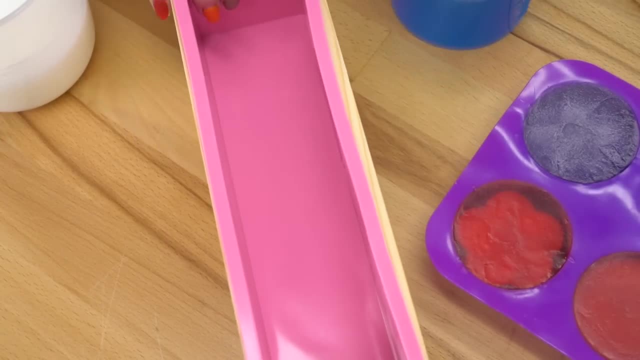 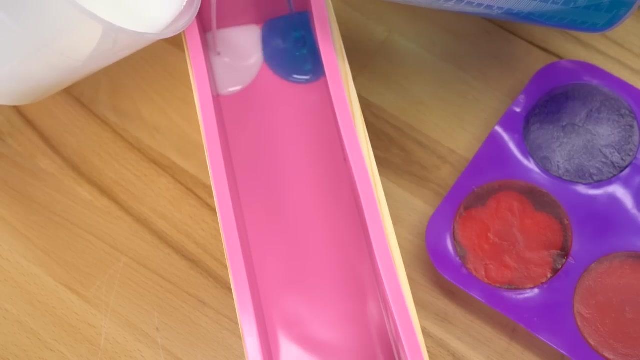 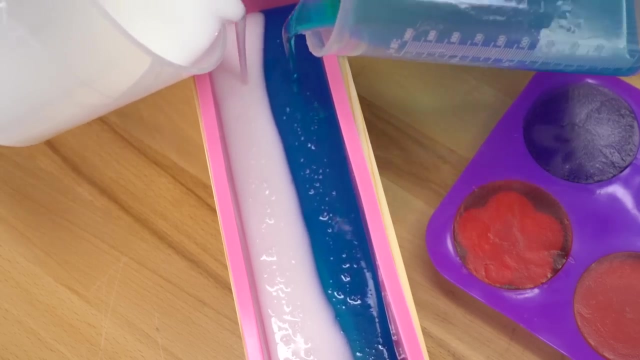 Let's test it and see how they do. Like what happens if we put our little mold here and then I pour them into either side? Are they going to stay separate? It looks like it. Okay, I'm just going to keep pouring because this looks so flippin' cool, Wow. Okay. well, this looks better. 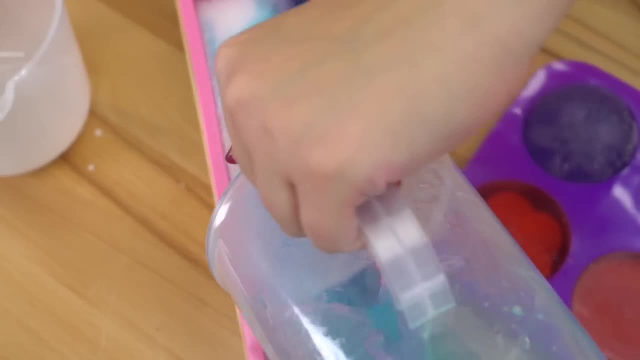 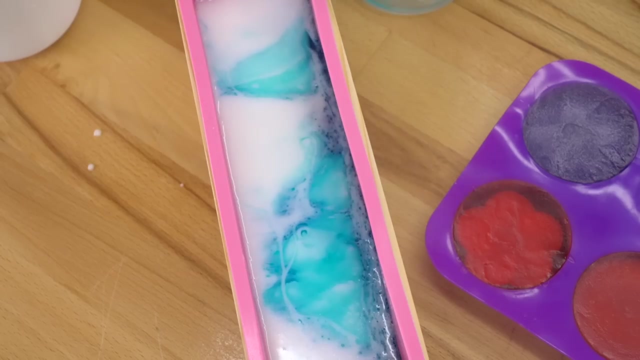 than I thought it was going to No lie. Get the rest of that blue out of there, All right, and I am going to just gently spritz the top. I don't want all that melt and pour to run away and get too mixed up. I just want those little bubbles to be popped so you don't need too much. 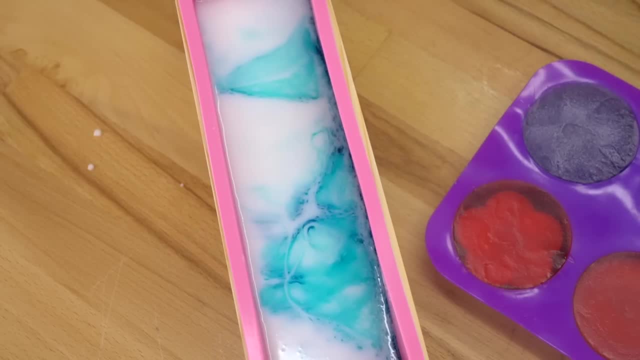 for that. That's it. I'm going to let that cool down a little bit and then I'm going to pour them into the mold That looks so good. I can only hope that it stays just like this, All right, and I'm just going to let it sit there for like 30 minutes or so so that I can come back and 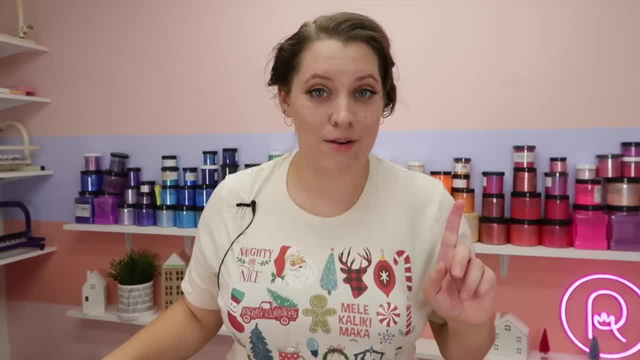 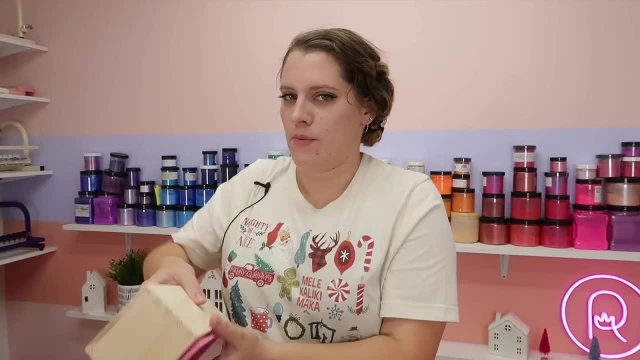 move all of these items out of the way. Okay, I'm back almost two hours later and, believe it or not, this is still warm, Like it is firm on top, but it's still warm. I don't think I can take it out of the mold. However, the purple ones are. 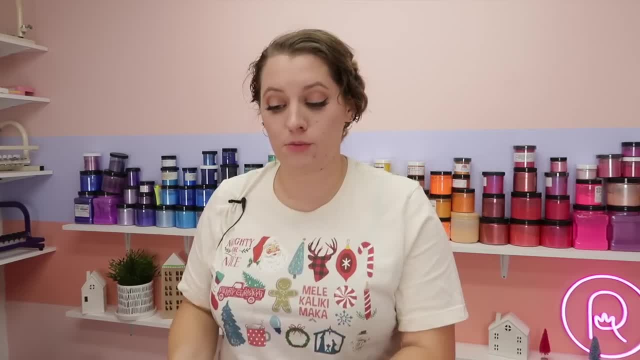 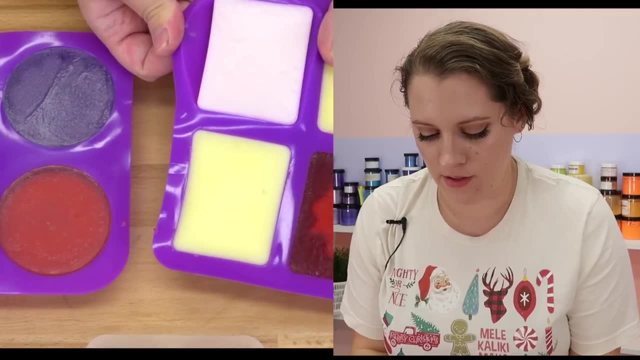 completely hard. They're so cute. Also, they smell really good. so let's go ahead and unmold those real quick. I'll start with the ones I poured first, which were the pink ones. Looks like they unmold pretty cleanly. Let's hope I don't pull the detail off. 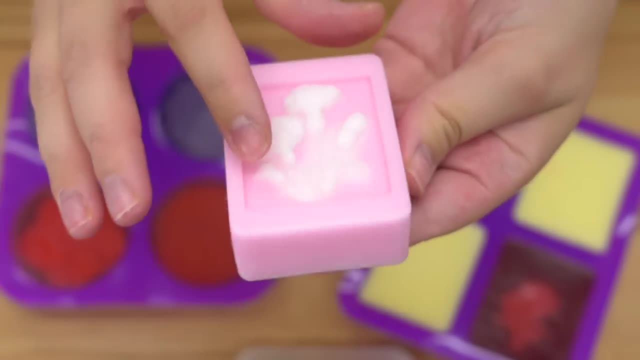 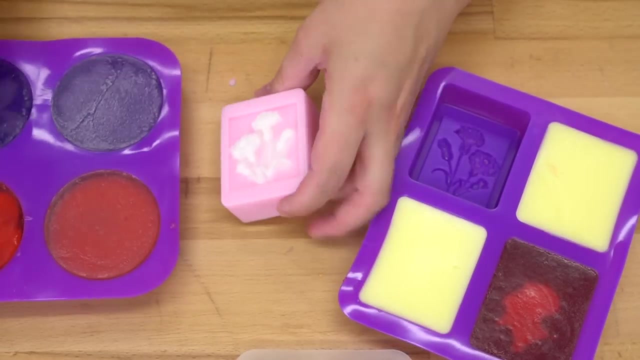 Look how pretty. So obviously we did have you know, a little bit of that white moving around, but it doesn't seem to matter. Like you totally get that those are flowers and reeds and stuff. It doesn't really matter that that smeared a little bit. Wow, it still looks. 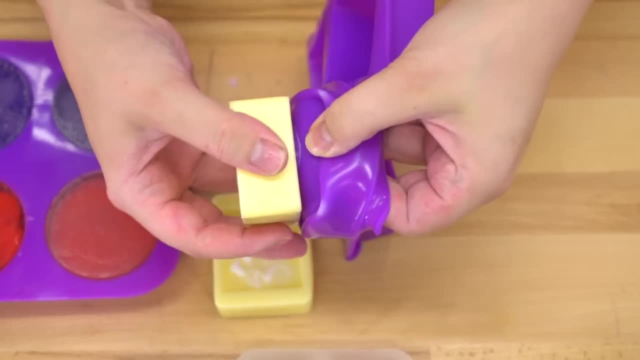 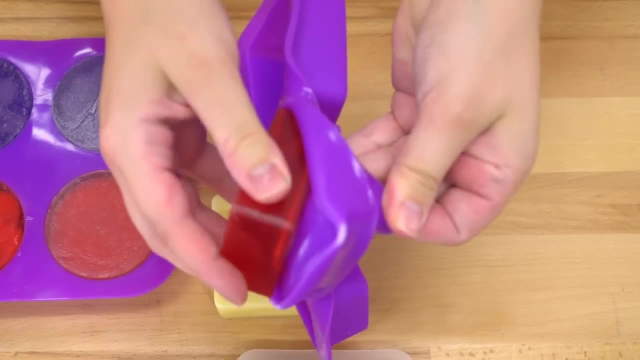 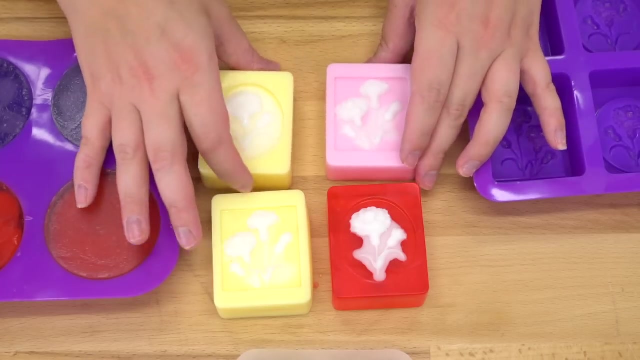 so good, though Very gently, because this one has the circle. Wow, so nice. And now for the clear red and white, which I think is going to be the most striking combination. Yes, these are so stunning. Let's go ahead and get some of the round ones out. So this one is our multi-layer. 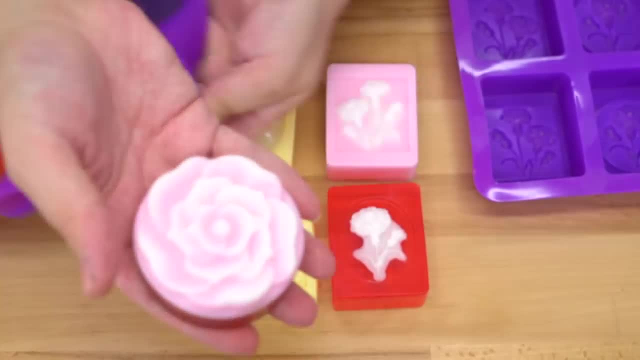 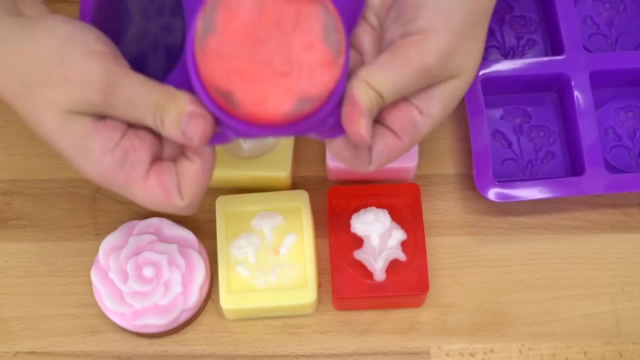 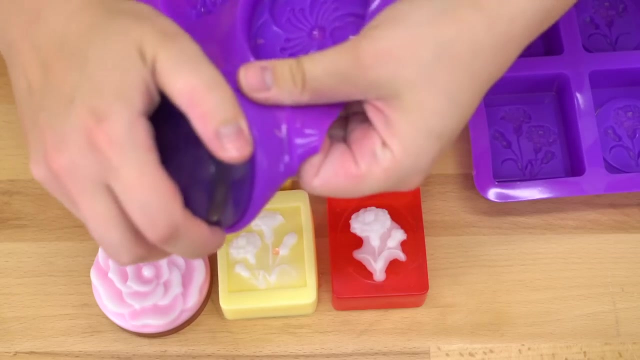 soap here that I kind of put all the extras in. Wow, look at that, though. That's so pretty. Like I said, the melt and pour really spread into all the areas you want it to Beautiful. These kind of look like something you might actually see in, like a little shop or something. I'm very 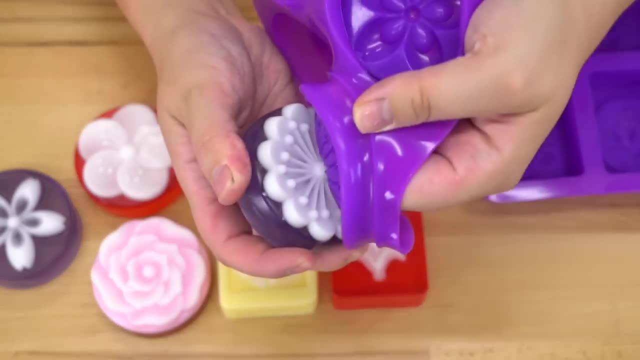 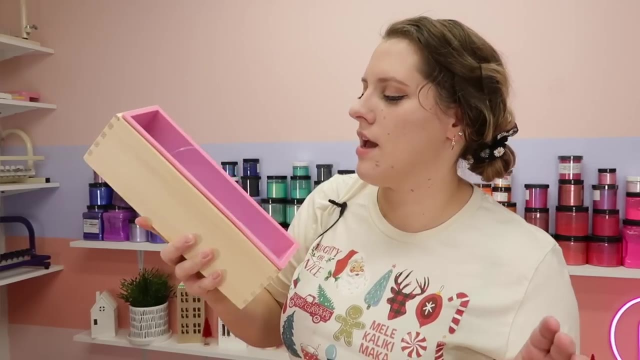 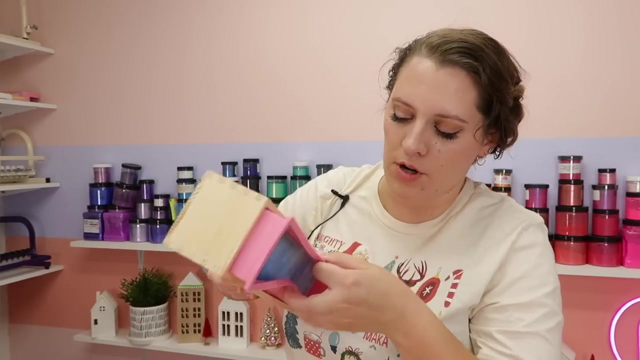 impressed. Look at her A little. last one here: So gorgeous. Look at these. Okay, but should we go ahead and just risk it anyway with this? I feel like we should Like. it doesn't feel like it's smushy, It's just still very warm. Will I be able to get it out? Okay? Is it firm? It feels firm. 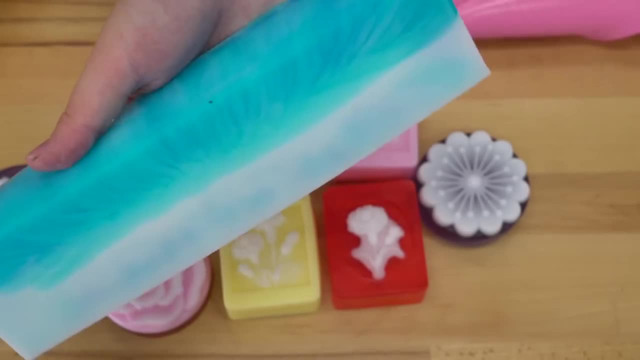 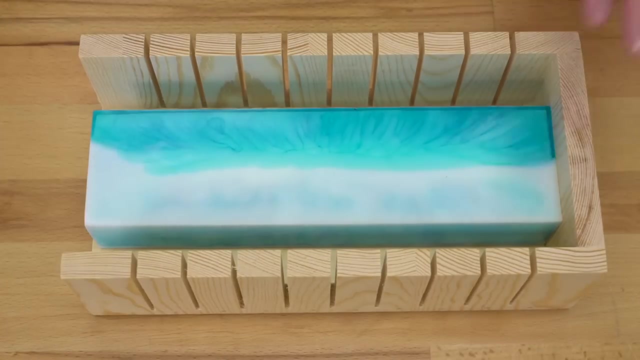 just warm. Look at this, you guys. That is so beautiful, That is so pretty Using our cutter here. I'm just going to line it up, I think, with the second one. Let's see, we'll start with the straight edge. We'll start with the straight edge. I'm just going to start with the straight edge. 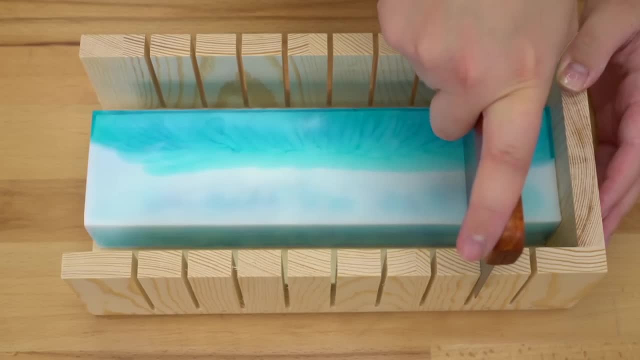 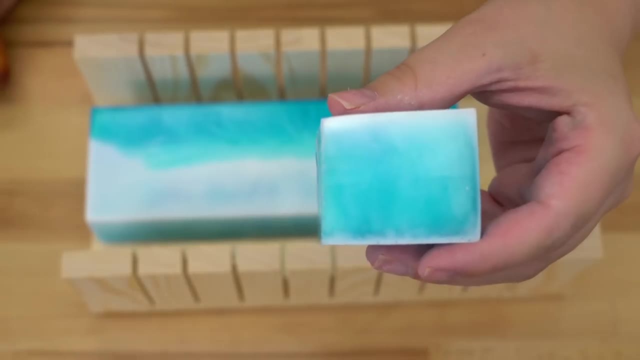 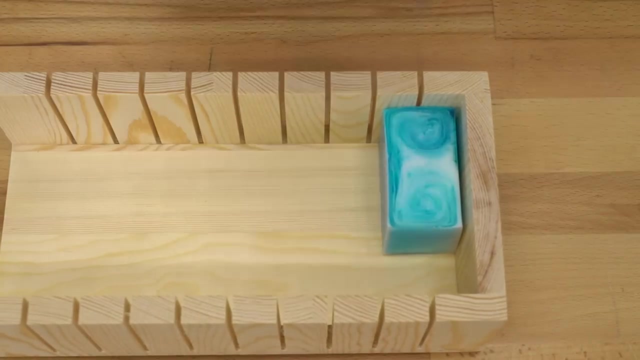 edge. I'm going to push as far to one side as I can so that, hopefully, I cut this pretty straight. How'd I do Pretty good, Pretty good, I'd say That's pretty straight. Look at that Gorgeous. Now I have pushed it to the very edge so that I can now cut this in half. I feel like I didn't. 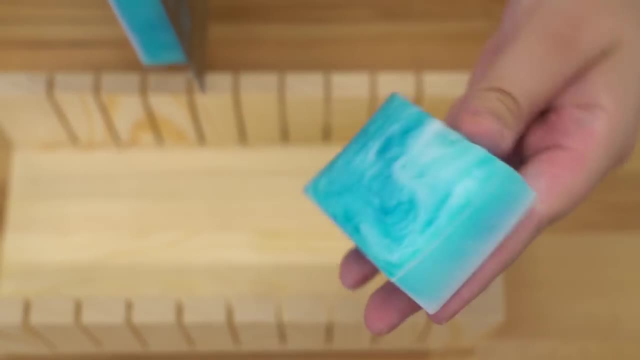 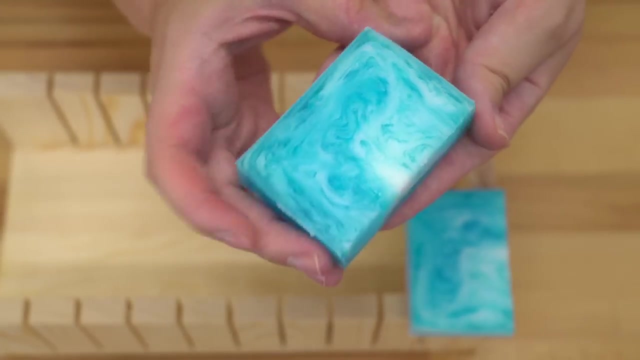 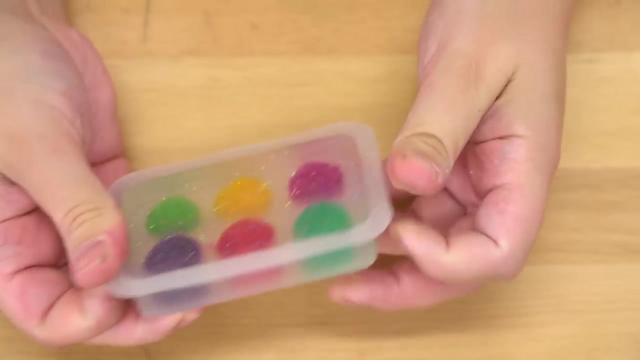 do as good on that one. Yeah, see, Sloped a little to the side there, but look how pretty the inside design is. I am obsessed. Okay, It has been over two hours at this point, so we're definitely ready to unmold our soap. I'm going to start by releasing the sides here. 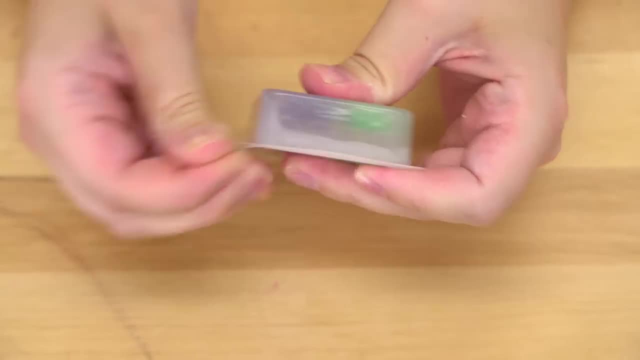 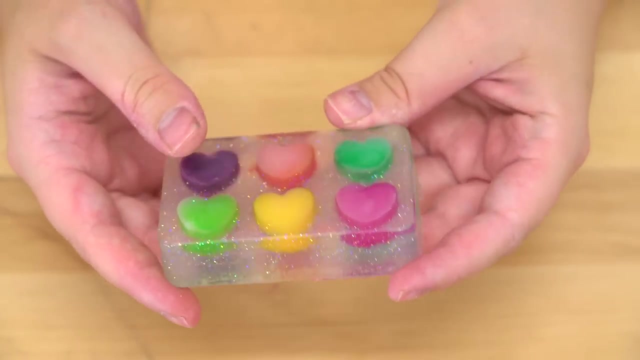 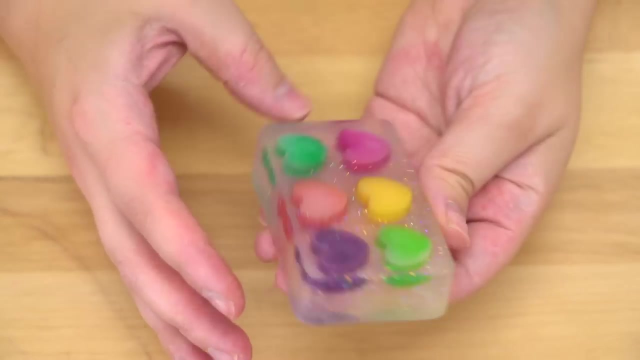 and then just pressing on one of the edges, And this is what it looks like on the inside. So I'm really impressed again by the clarity of the melt and pour It looks, looks so good. The sparkles are super, super pretty and then, of course, it's just the perfect shape for. 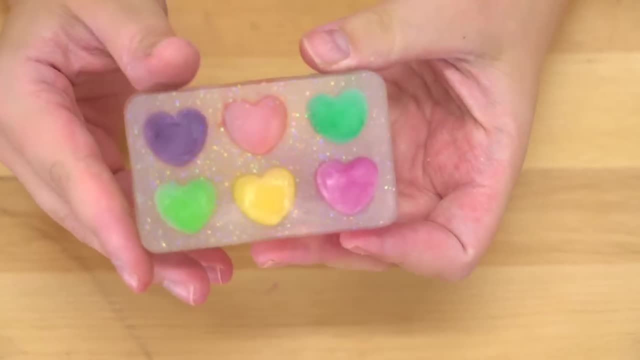 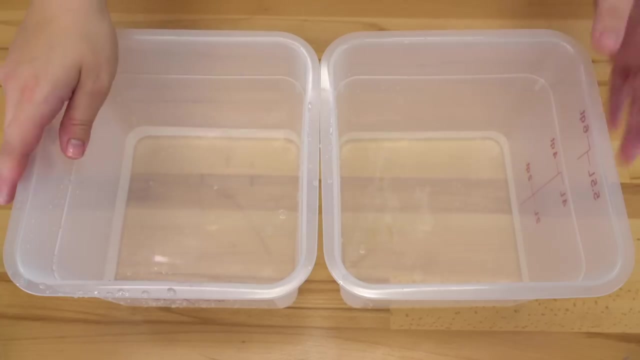 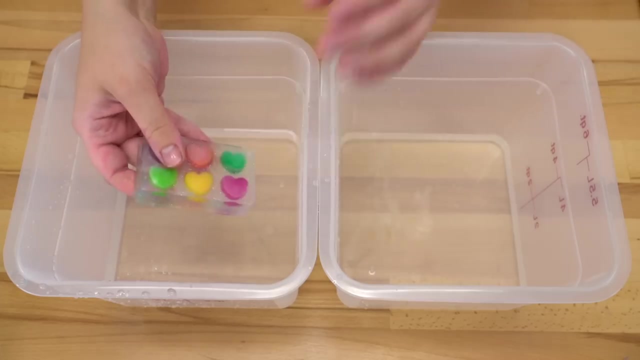 little hands, Still a little disappointed that it doesn't smell. but for nine dollars getting to make three of these, that's. that's pretty good. Now that I have unmolded and cut both of our soap kits, it's time to see how do they perform. We'll start with our cheap soap. So first of all, looks even. 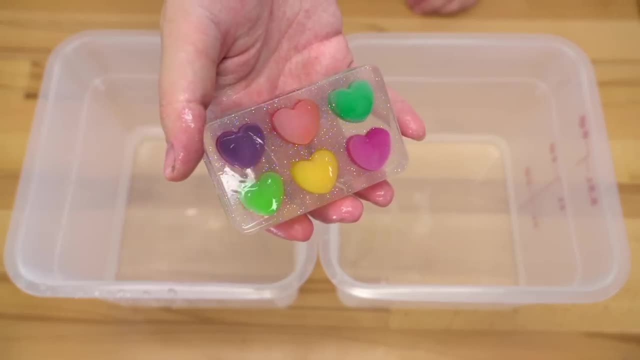 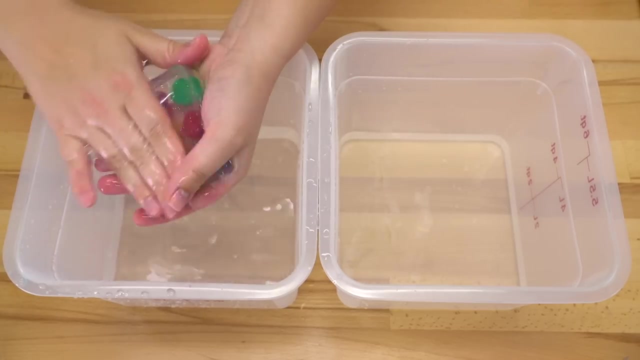 better when you get it wet. You see, adds to the clarity Any tiny bit of cloudiness just leaves. I will get both of my hands wet here. I'm not feeling any grit from that glitter like I thought I might, and it lathers very, very decently. If I was a child and I made this kit, I would 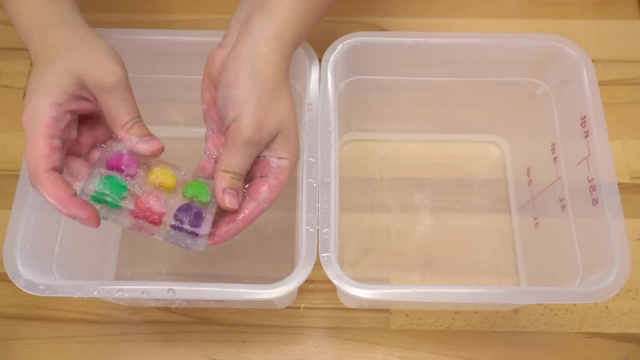 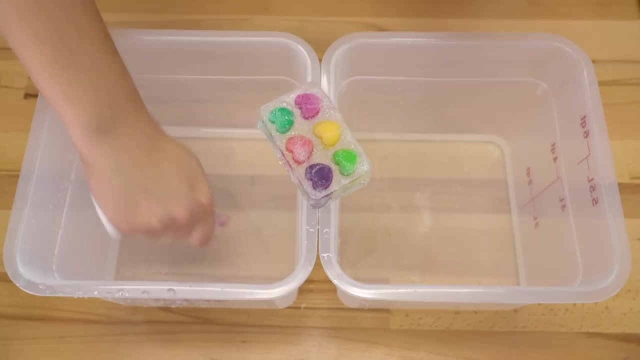 be pleased as far as, like the usability of the soap goes Very fluffy, very bubbly, very soft, Like it's just it's a really good lather and sometimes with these cheaper craft kits the melt and pour is just awful, Like it just doesn't lather at all. but that doesn't seem to be the case. 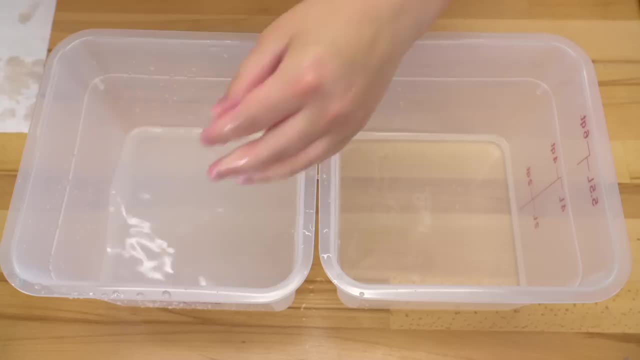 with this one. It works really well. Okay, gonna dry my hands in between washings so I don't have any extra residue Left on my hands. and let's see, let's go for our purple, Our purple one here. That looks pretty. 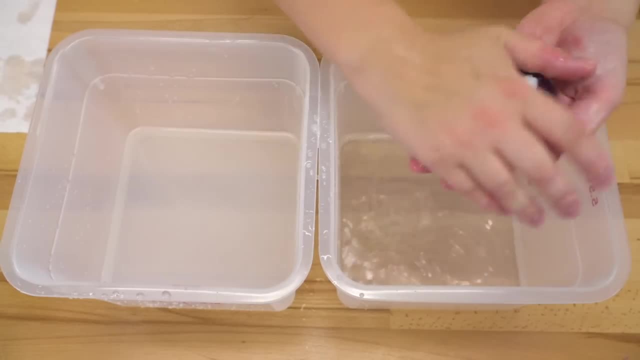 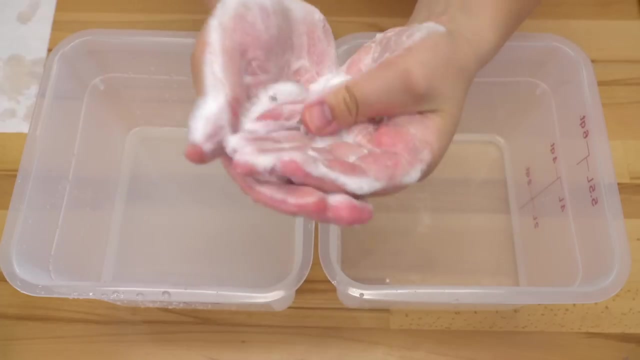 This one also has enhanced clarity once you add it to water, and it also bubbles very well. I think it also helps that a lot of these soaps here have some ridges and some bumps. That always helps create lather. Yeah, lather is super good. In fact, I would say this one is even a bit more bubbly than 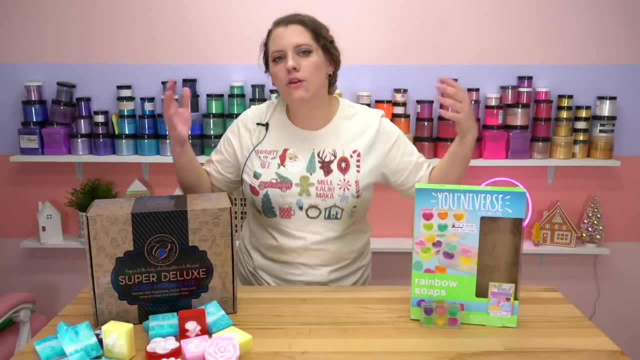 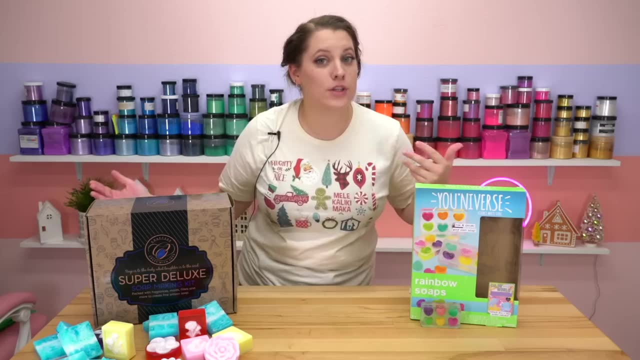 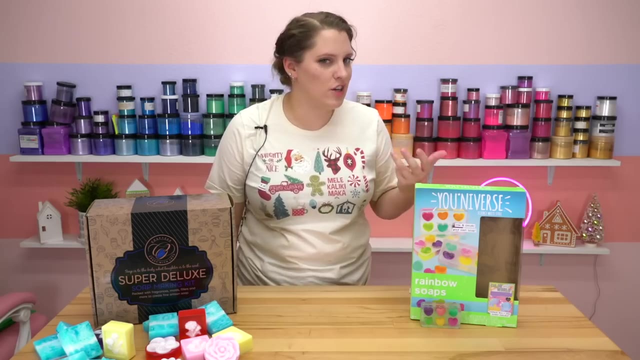 the other one. Okay, so what are my final thoughts and my conclusion about the expensive soap kit versus the cheap one? Well, I have some critiques for both kits. For the cheaper one I would say no. fragrance oil is a big turnoff to me personally. You cannot achieve the colors that they advertise. 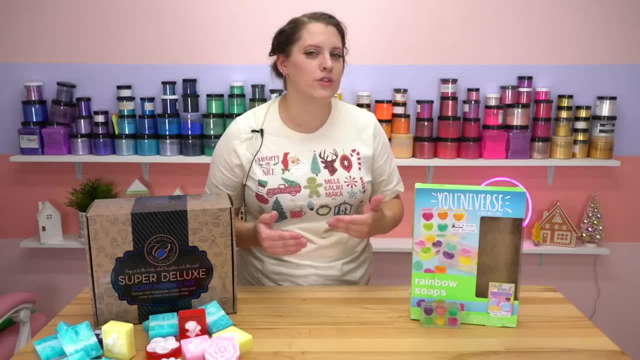 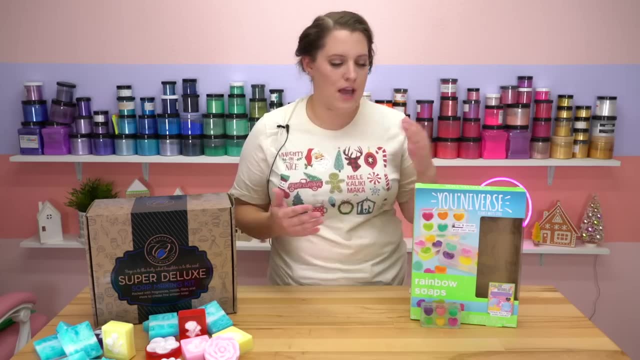 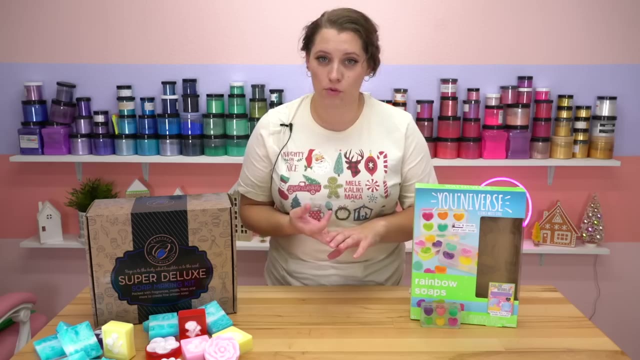 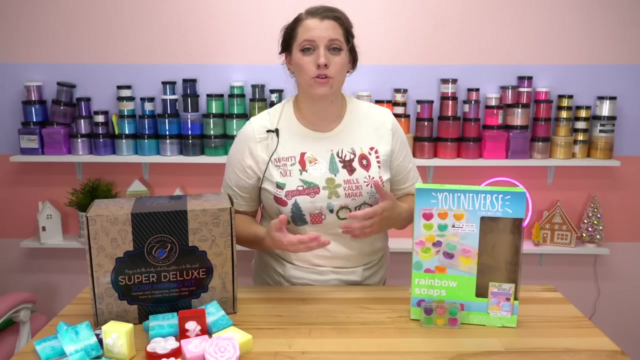 on the front of the box, and it is pretty difficult to mix up those embed colors the way they request that you do. I would also add some extra materials. The extra materials I would recommend you use if you buy this kit are a toothpick, a popsicle stick and some rubbing alcohol. Most of those things you can get at Walmart or a local drug store, so it's not a big deal, but it is still something you will have to supplement in addition to this kit to make it work the best it possibly can. 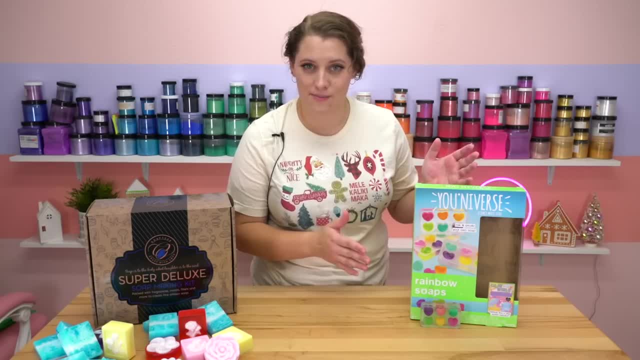 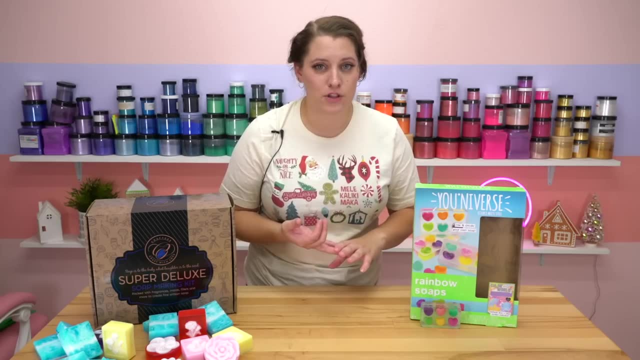 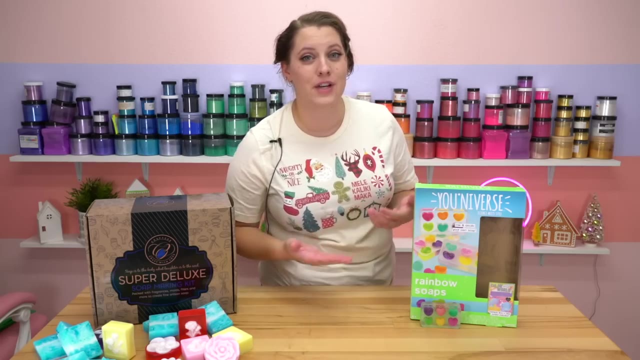 In the future. I would also love to see the glitter be eco-friendly. but those were my main issues with the kit. The color pigmentation was really good, The clarity of the melt and pour was really good, The soap quality was really good and you get to make three soaps for $9, so around $3 a piece, which is very, very inexpensive for a craft kit. 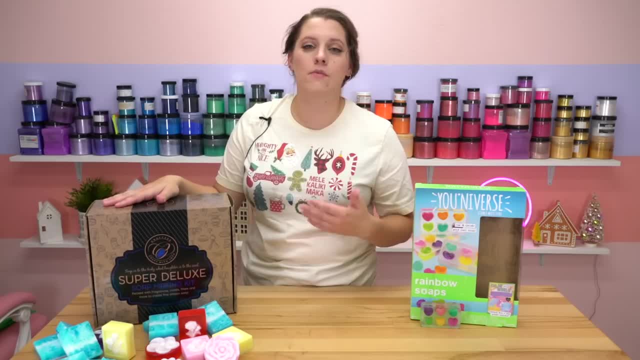 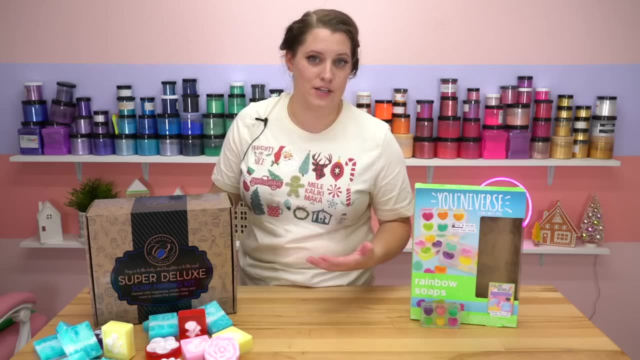 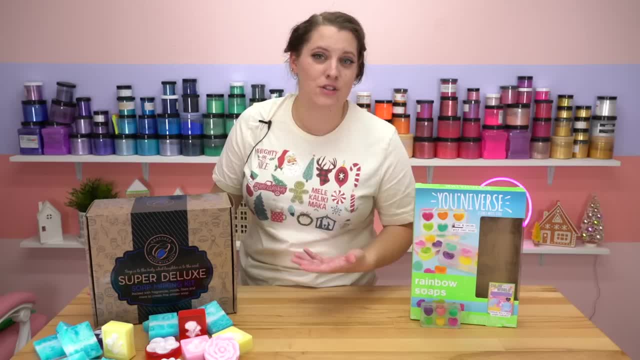 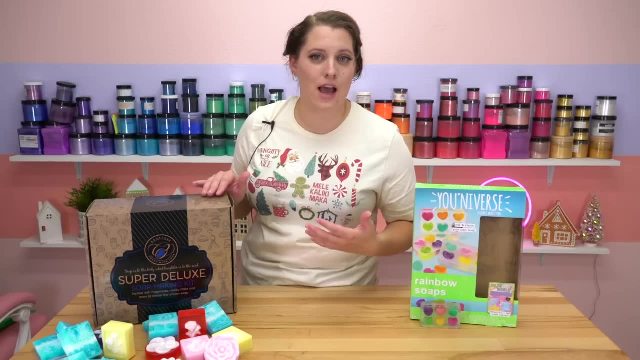 One that is easier to incorporate into the product. One that is easier to incorporate into the product. Flowers look bad in melt and pour after about 24 hours. I feel like a lot of what made this particular kit the price that it is had to do with including the miter box and the two cutters. 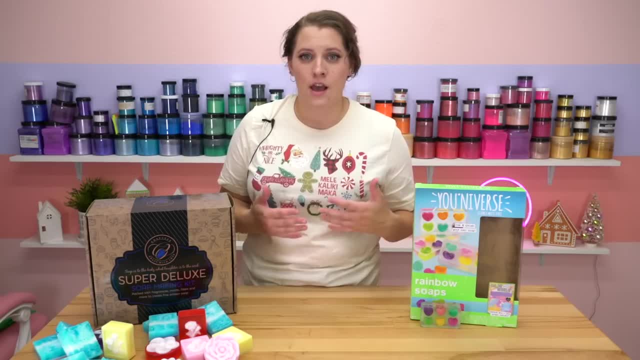 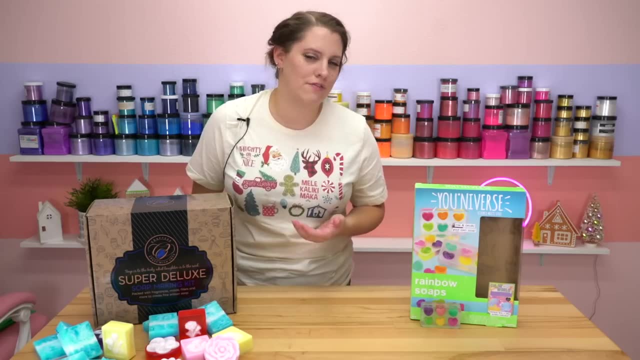 Neither one of those things are things that I think are necessary, and I would feel better getting to purchase a kit without those options. that was a lot cheaper, because they're just not effective in my personal opinion, and I never recommend them to people who are not going to use them. 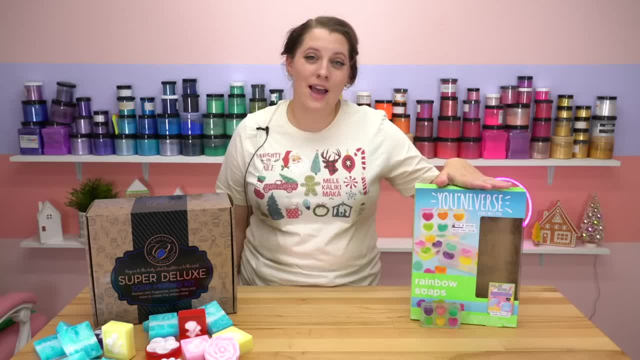 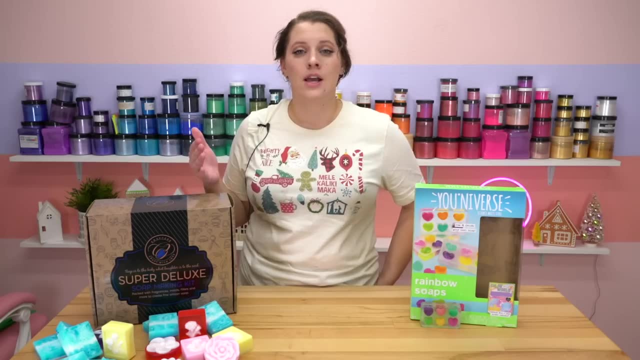 Neither one of those things are things that I think are necessary, and I never recommend them to people who are not going to use them. With this kit, I had to add rubbing alcohol, a toothpick and a popsicle stick. With this kit, you really just need extra rubbing alcohol and a sharp knife, which you kind of need for this one because you have to cut up soap either way. 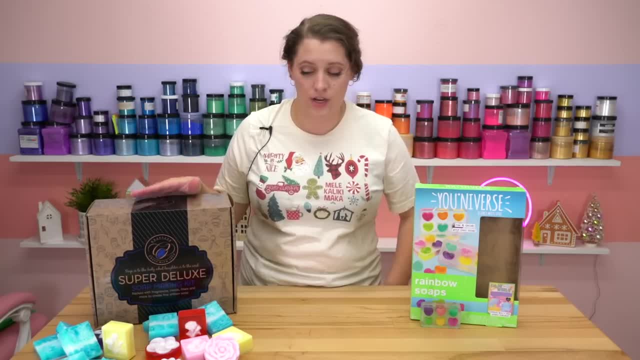 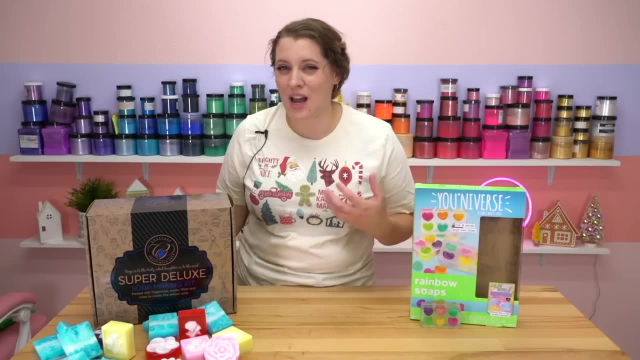 So less to add as far as this one is concerned. And then the other critique that I have is the fragrances. A lot of the fragrances are in the same kind of scent family and they smell very powdery to me. So less to add as far as this one is concerned. And then the other critique that I have is the fragrances. A lot of the fragrances are in the same kind of scent family and they smell very powdery to me. 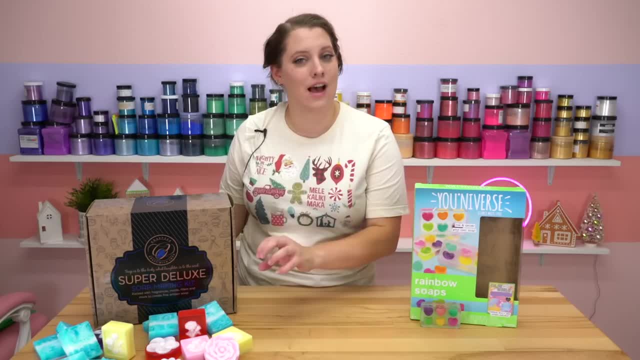 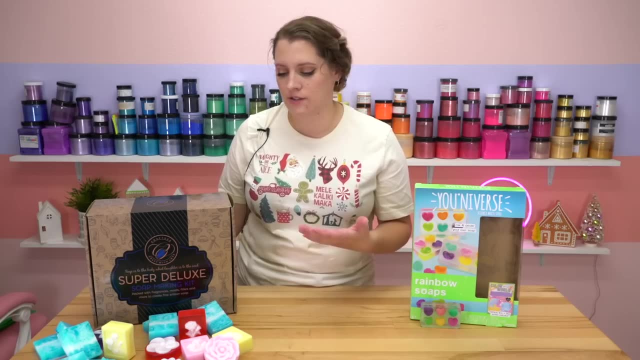 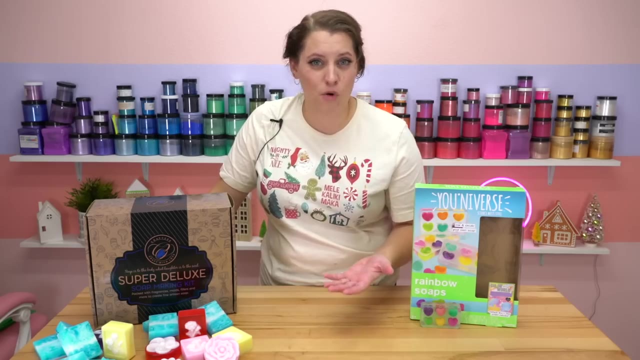 I personally feel like they match the designs on the silicone molds. So it's sort of an older, perhaps more mature scent. It's a little more powdery. The color pigmentation is great. The amount of soap that you get in this kit is great. It's like 4 lbs, which is quite a lot. 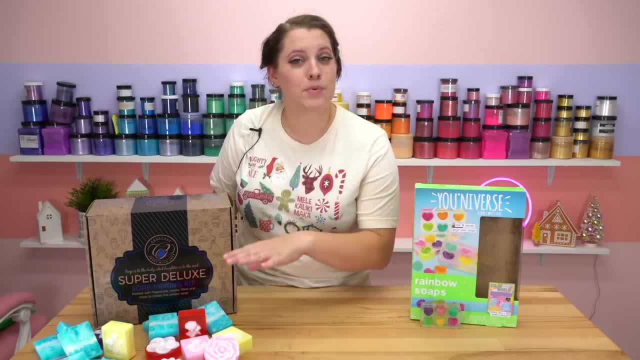 Now, the last thing that I will say as a critique for this particular kit is that you could probably get 4 lbs of melt and pour. Now, the last thing that I will say as a critique for this particular kit is that you could probably get 4 lbs of melt and pour. 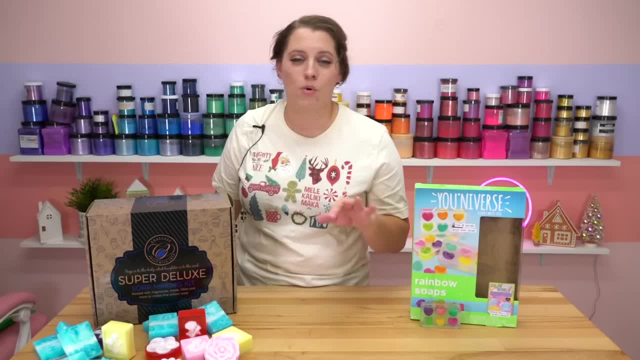 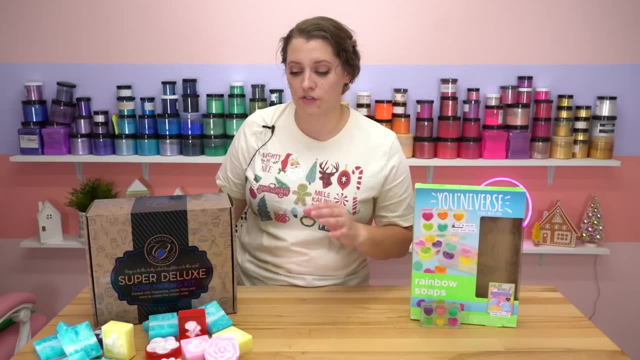 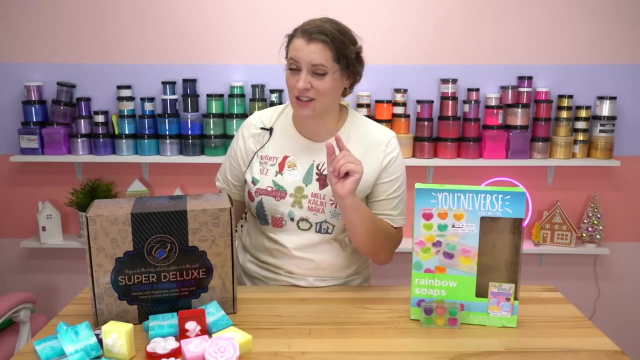 whatever colors you personally prefer, One or two fragrances on Amazon in its own little kit and whatever mold you personally prefer, for cheaper than $80.. I don't know for sure, I'm just saying that's my guess. So I do feel like this is just a smidge overpriced and I wish it. 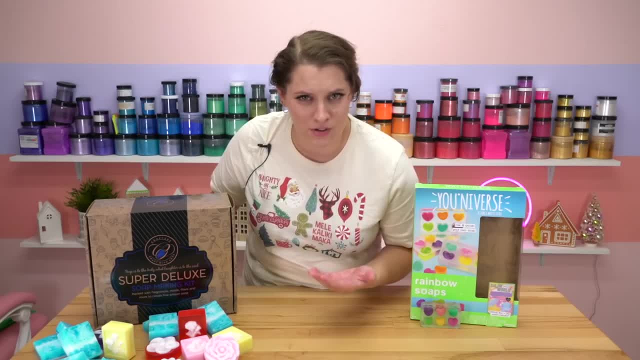 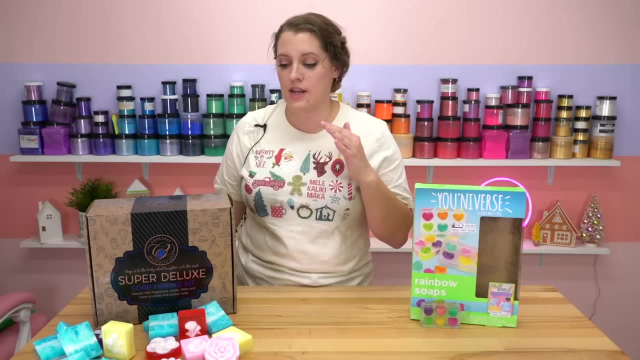 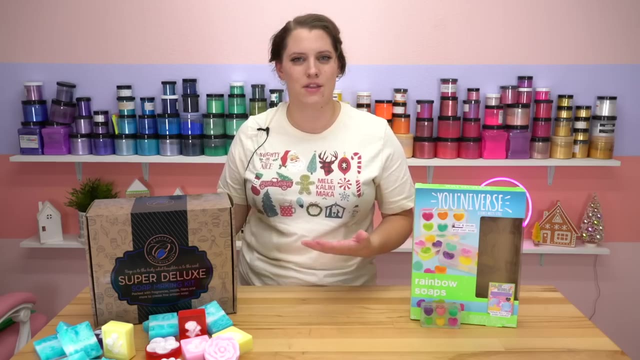 didn't include those other items. However, that is my personal opinion. If you really love to use a box and a wavy length cutter- and that is your jam- then it is a very good price and well worth your money. It is very, very detailed. It's put together in such a way that I think is nice. 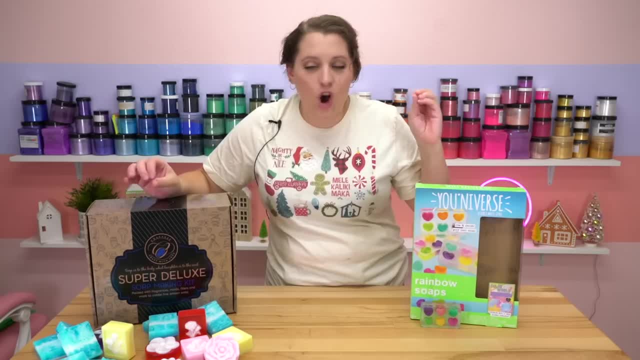 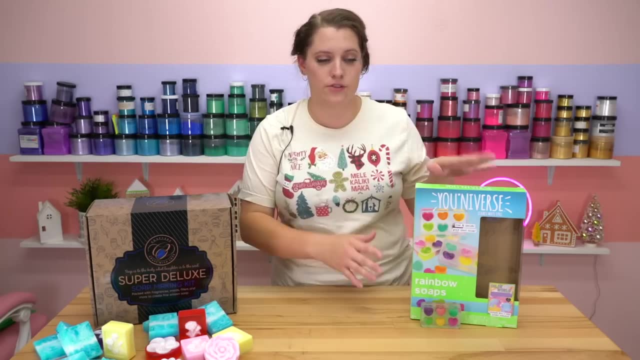 So who wins? That's the real question. It's hard to say because I kind of am comparing apples and oranges here. This is clearly targeted to adults. This is clearly a child's kit, but I would plunk down another $9 like that. 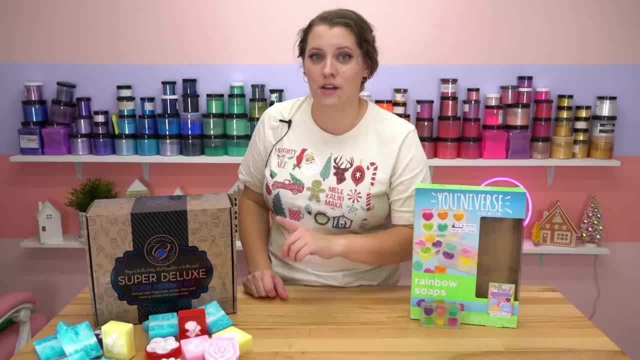 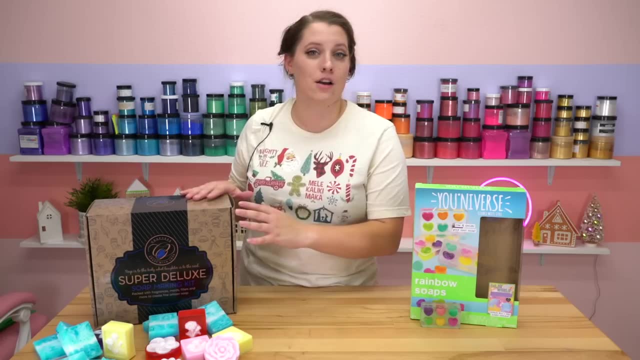 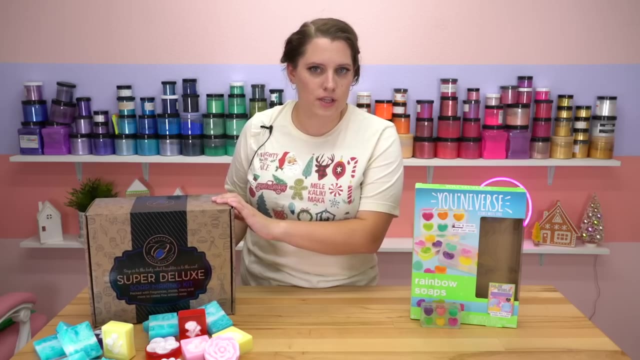 I would hesitate to spend another $80 on this kit just because I trust my own ability to source these materials cheaper. That's not a knock on the kit. It is just saying that I think I could get it less expensively if I shopped a little more. This is a great option. It really is, And it doesn't. 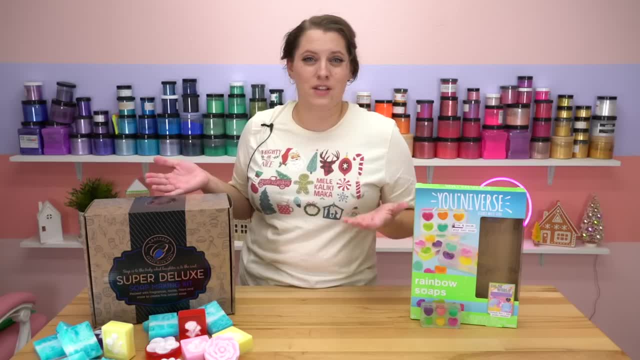 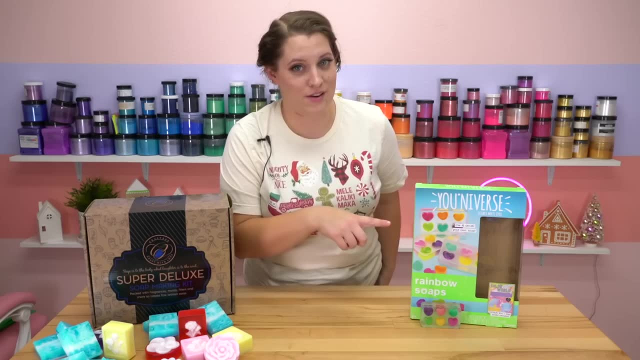 have any lye in it, So it's also something that's relatively safe. You know, I really I like them both, but I would buy this one again- as a soap maker myself, Personally and if you're watching this, so that you can buy something for grandkids. 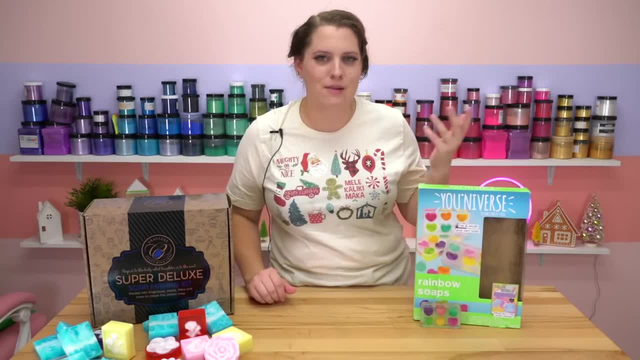 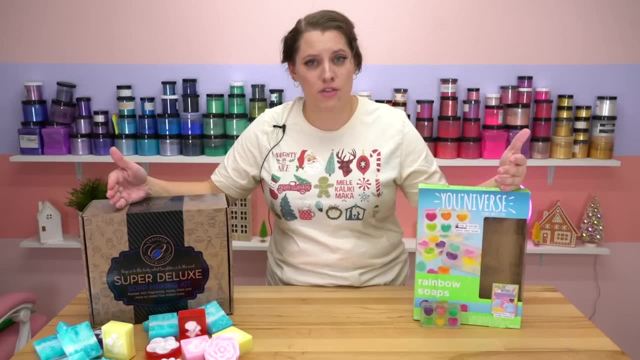 spend nine and then maybe buy one or two of them and they can make six soaps and that's plenty for any kids. So those are my final thoughts and conclusions. Both of these are great, Both of these are worth purchasing. I will leave links to them down below. This has been a really really 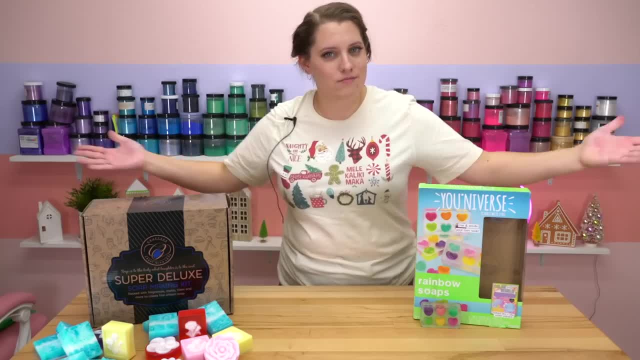 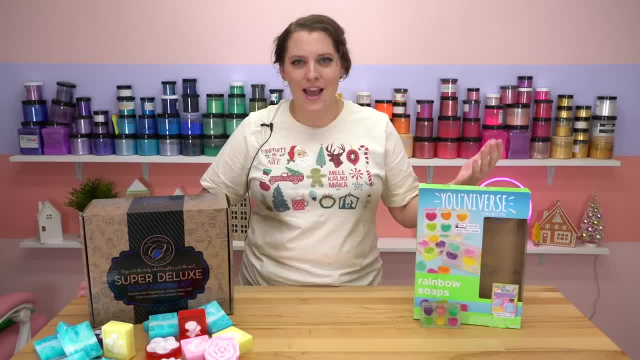 I love to see which videos you guys prefer that I make and, yeah, have an absolutely royal day. I'll see you in the next soapmas video And until then, bye for now. Give this problem a try and, when you're ready, keep watching the video for the solution. One way to solve this problem is by using several geometric principles. One principle is that a straight line measures 180 degrees. We can look at the angle next to.